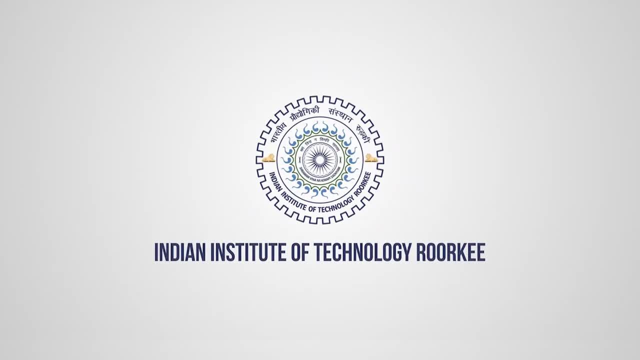 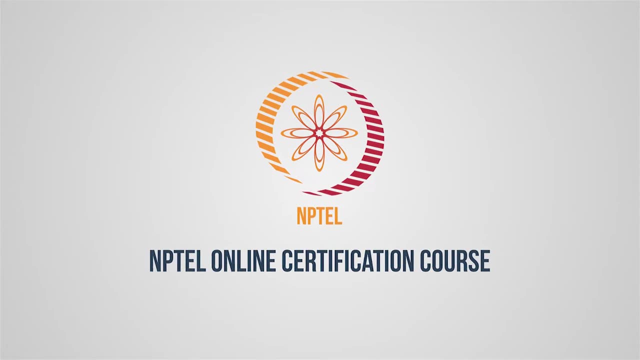 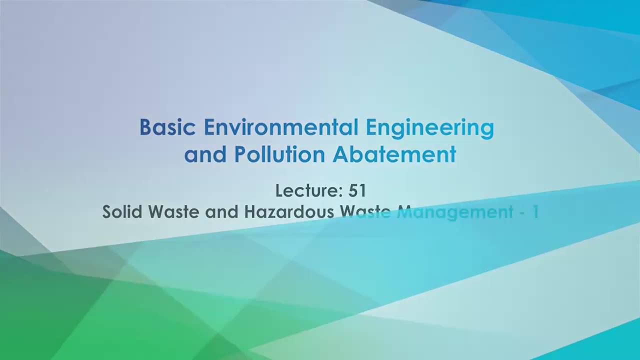 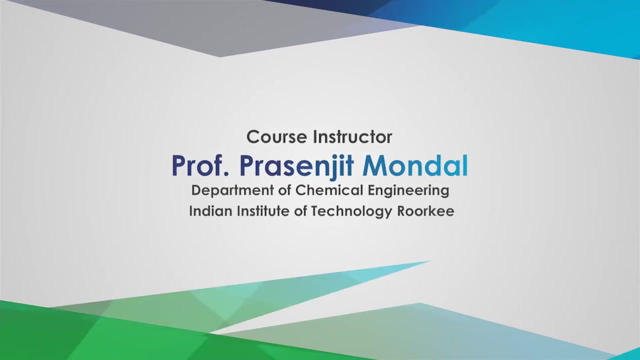 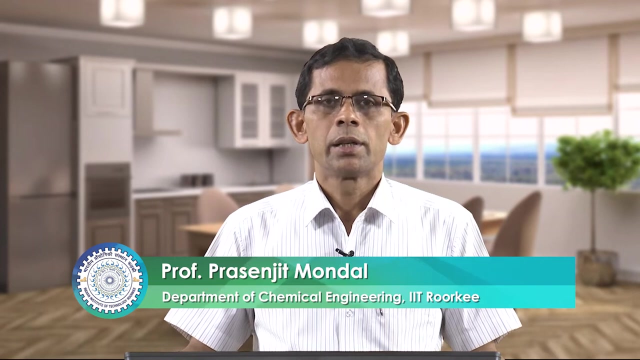 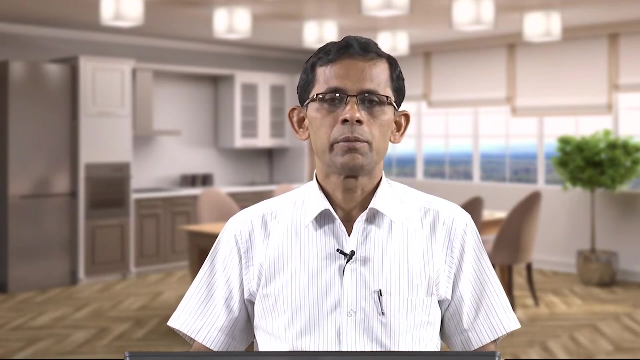 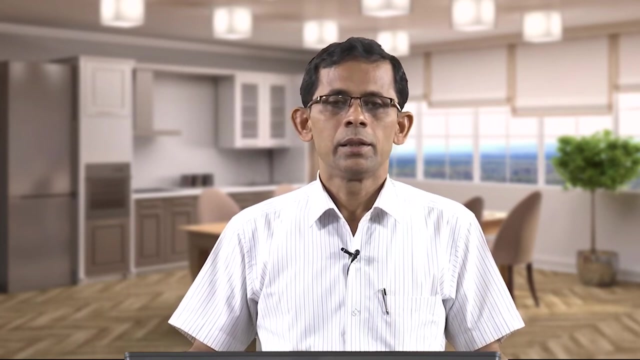 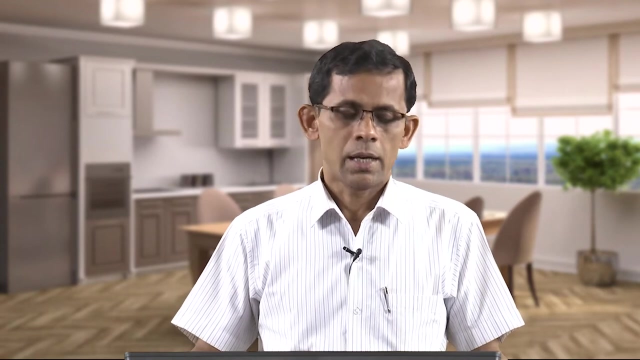 Hello everyone. now we will discuss on the topic solid waste and hazardous waste management, part 1.. Already we have discussed on the management and treatment of different type of waste streams like air, water, and the next part is with solid waste and the hazardous waste, and the contents are: classification of solid waste. 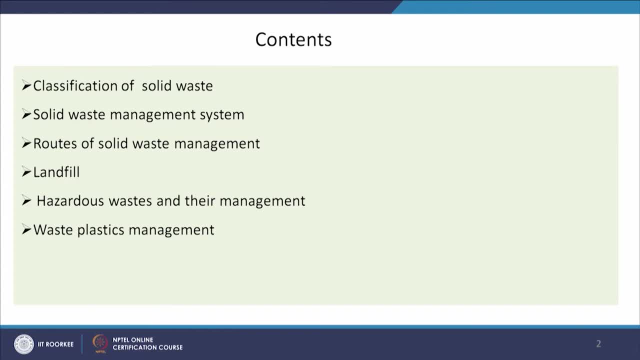 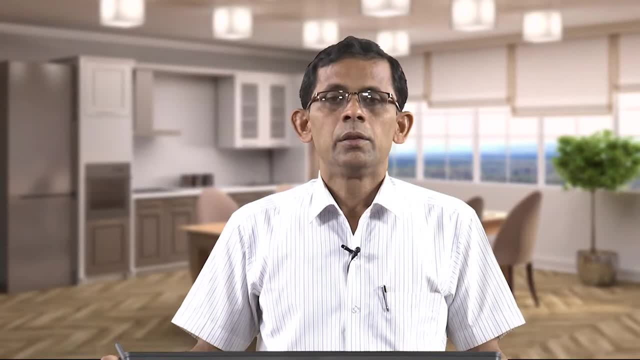 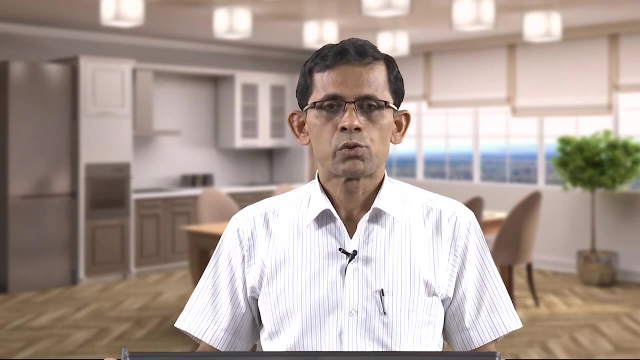 solid waste management system. roots of solid waste management, land filling, hazardous waste and their management, and waste plastics management. Now we will see the classification of solid waste. So the name itself indicates that the waste will be in solid phase or solid. 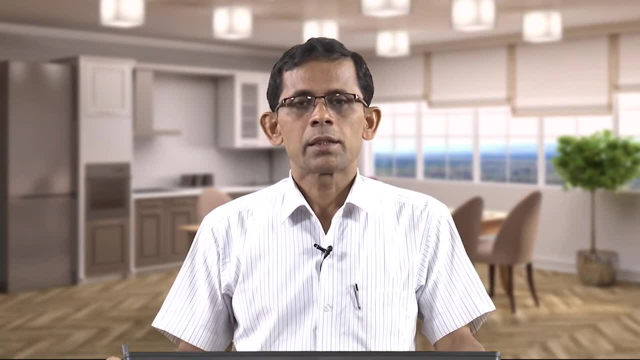 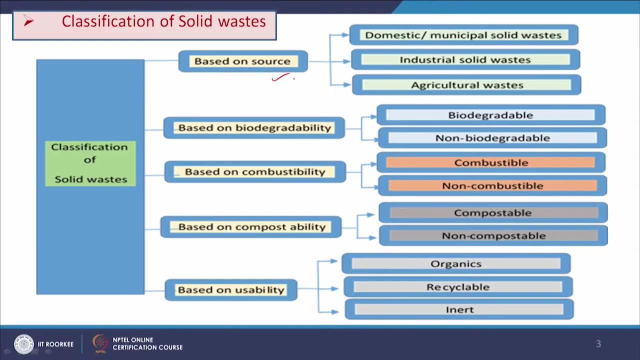 state. So we can classify the solid waste based on some criteria like, say, based on source: it can come from domestic or municipal sources, it can come from industrial sources or may it come from the forest. So industrial solid waste, agricultural wastes and domestic and 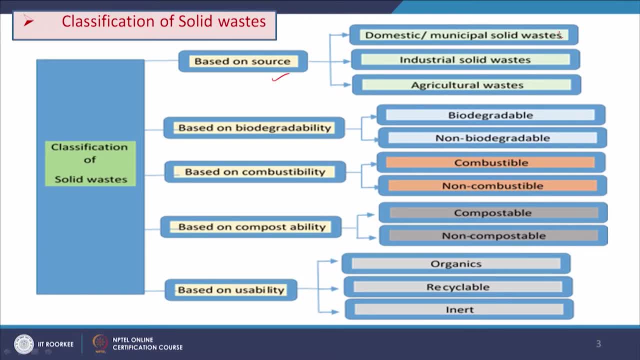 municipal solid waste. that can be the classification that agricultural and forest waste are under the same category and, based on biodegradability, this can be biodegradable and non-biodegradable and, based on combustibility, may be combustible and non-combustible. 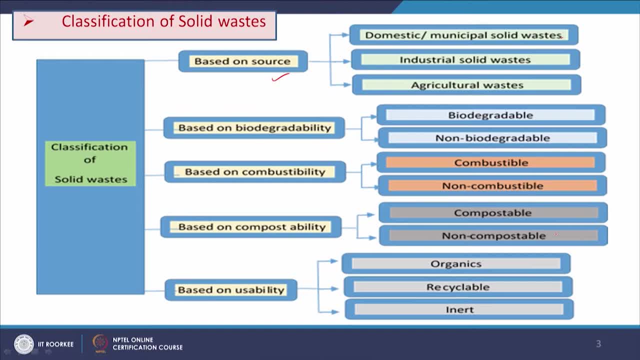 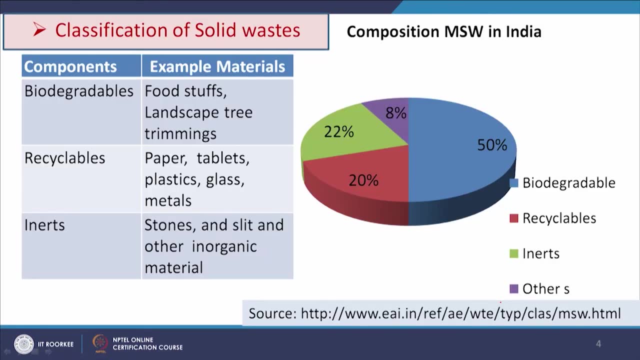 And based on compostability- that is, compostable and non-compostable. and based on usability- that can be organics, recyclable and inert. So these are the different types of classification of solid waste. Now we will see the characteristics of municipal. 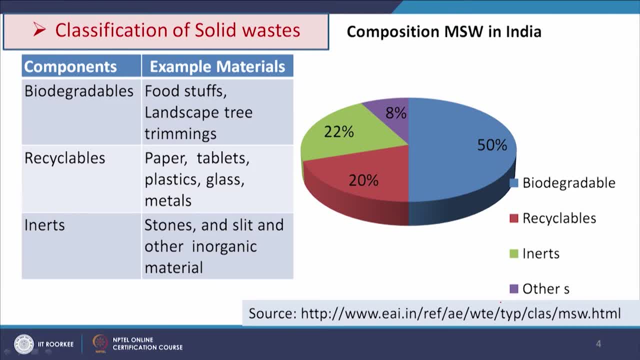 solid waste. So municipal solid waste, if we see around 50 percent contains biodegradable material and around 20 percent contains biodegradable material. So this is the classification of municipal solid waste. So municipal solid waste, if we see around 50 percent contains. 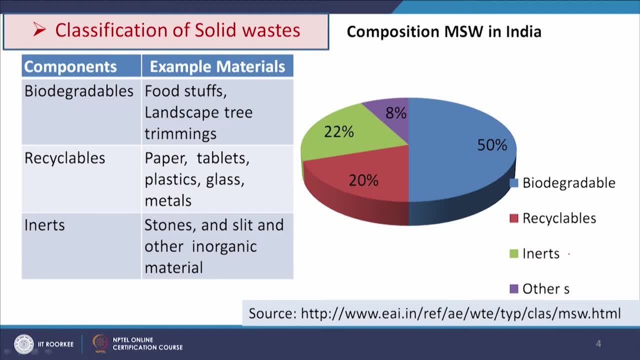 recyclable materials and around 22 percent inert material, and 8 percent is others. Now we will see that biodegradables may be the foodstuffs, landscape treatments, and recyclables may be paper tablets, plastics, glass, metals, etcetera, and inert may be stones and silt. 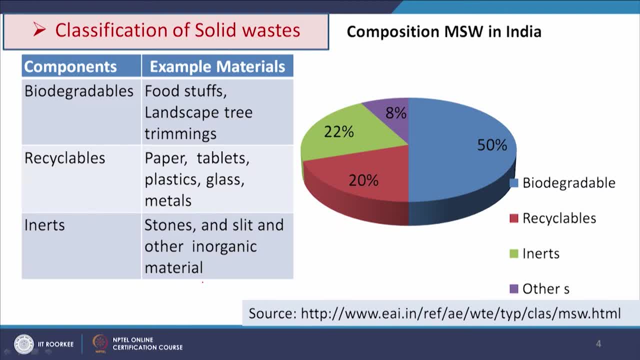 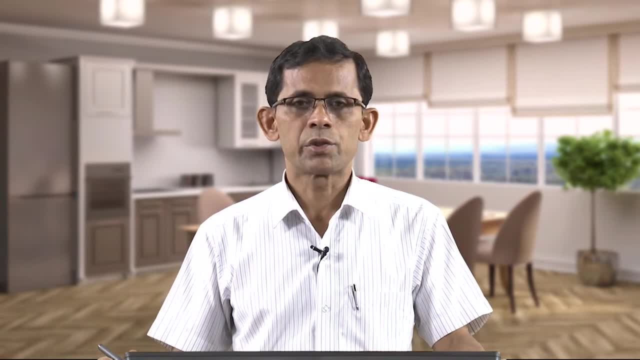 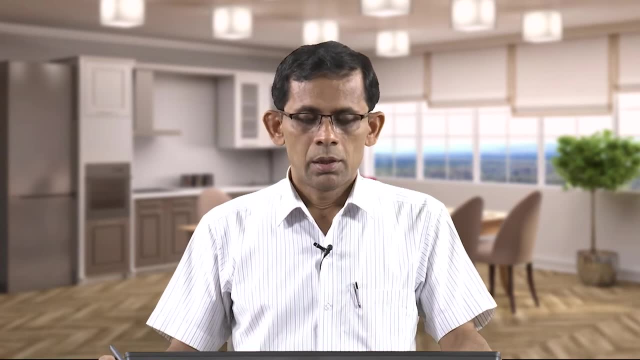 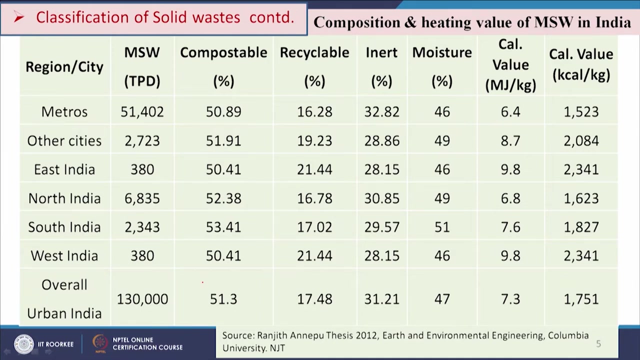 and other inorganic material that is, construction debris, etcetera. So these are the different components which is available in the municipal solid waste and their relative contributions on the overall volume of the MSW. Here we will see the source of MSW from different parts of the country and their composition and some characteristics. 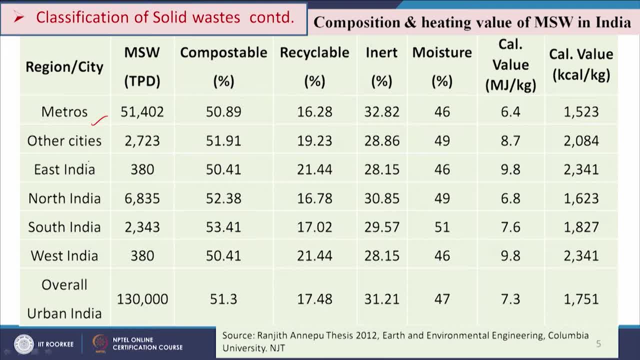 like, say, if we see metros, metro cities and other cities and East India, North India, South India, West India, India, if we classify these and if we see the municipal solid waste, So their concentration of different types of materials will be different and their properties will also be particularly. 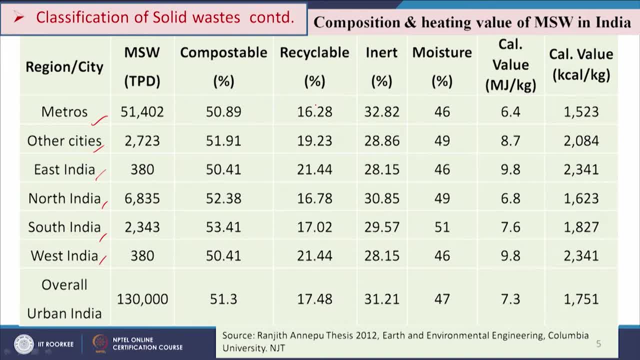 the heating value and moisture content will also be different, And this table shows us some example case study that is based on 2012 study. So these are the total production in ton per day and these are the compostable present in it. So 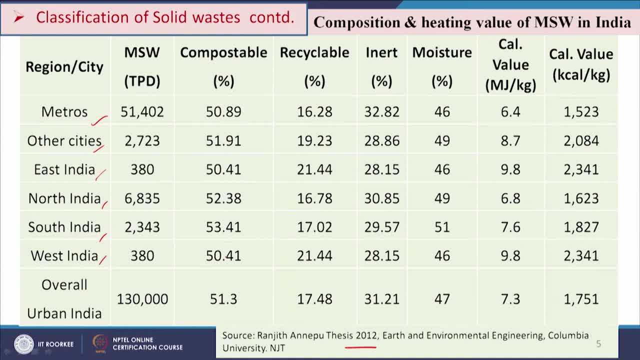 it is evident that around 50 percent plus minus some compostable material is available in the MSW, produced in the different part of the country, And recyclable materials also say 16 to 21.44 percent is mentioned here. So around 20 percent we can say, or 22 percent. 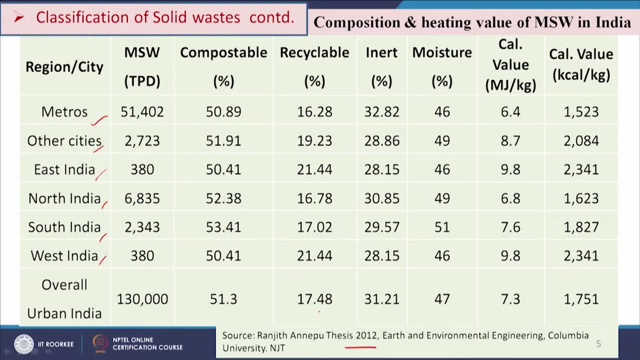 we can say that Recyclable is there maximum. So inert is also present. there you see 32.82 and somewhere it is 29, like this. So that way inert material is also present and moisture content is also mentioned and calorific value we see. So calorific value is not very high, but it can. 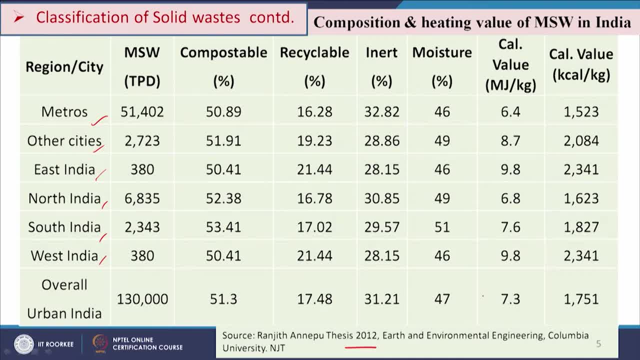 be recovered. So this is the characteristics of MSW available in the country Now the, although the calorific value is less, we see here. but if you can segregate the different components, because you have seen that here, inert is around 20 to 28 somewhere. 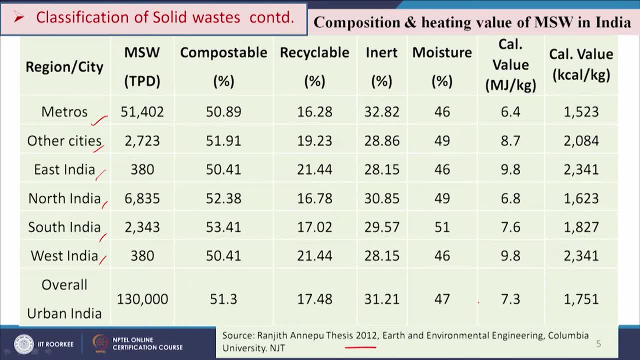 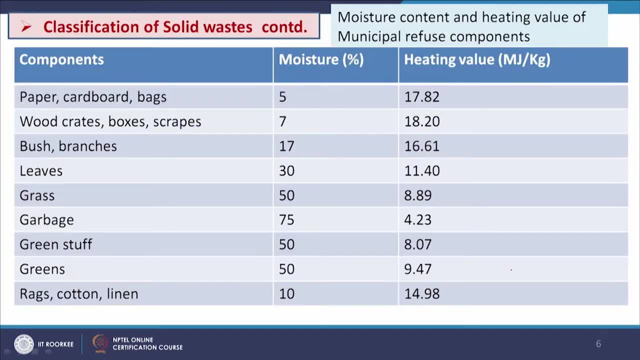 32 percent somewhere. So if we can eliminate this part, So this, your calorific value will be increased. So segregation of MSW, if you can do, then the particular fractions we can get that can have very high heating value. And the other thing is that if you can segregate, 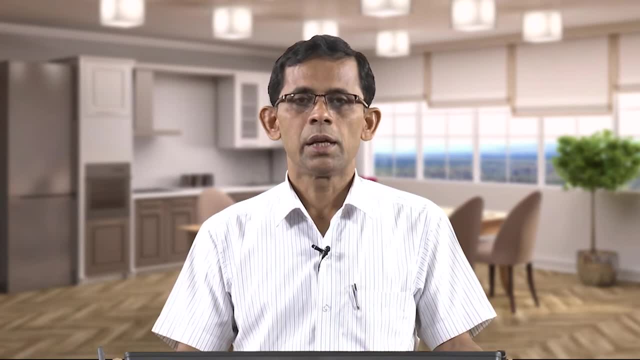 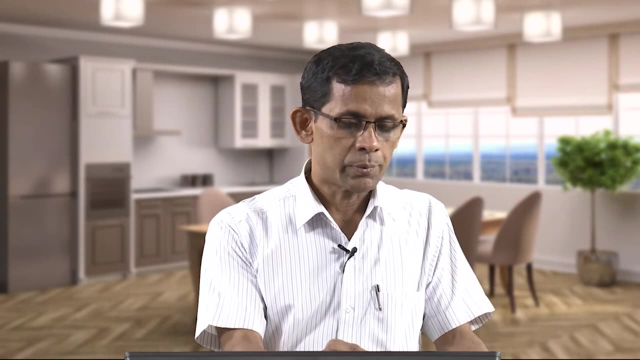 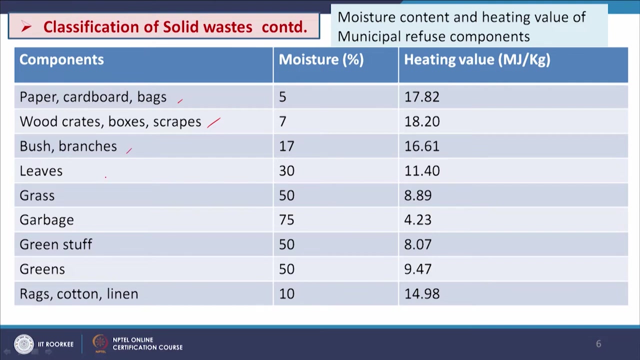 which is the these. Heating value is also varying widely. that is 4.23 mega joule per kg to maximum. it is mentioned here 18.20 mega joule per kg. So 18.20 mega joule per kg is a good amount of. 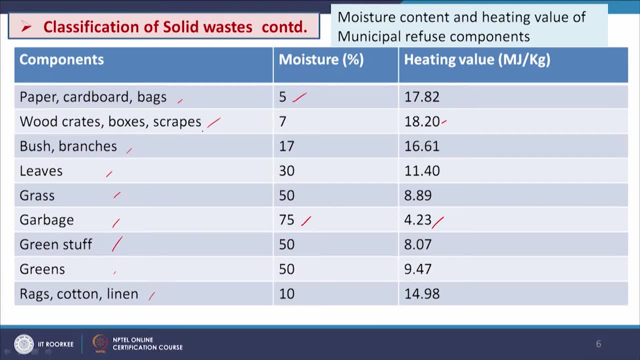 heat content this type of materials is having, So this can be used for the energy recovery. but where are these materials? the? although the heating content is less but its moisture content is high, So this can also be treated biologically for the recovery of the energy. 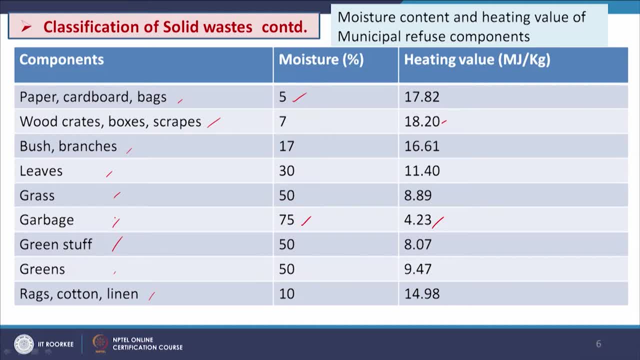 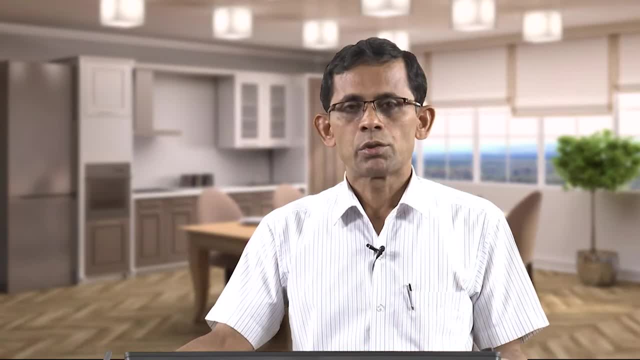 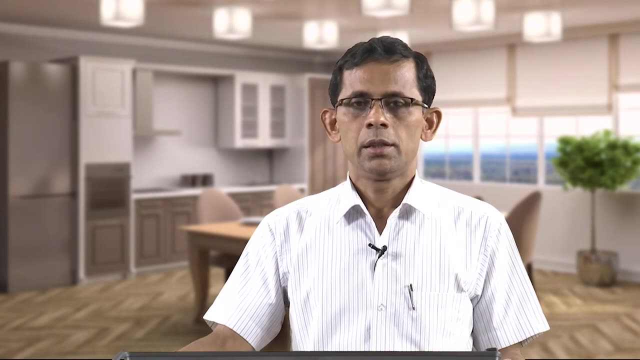 or the production of biogas, and overall value addition can be taken place through the treatment Similar to MSW. the industrial solid waste will also contain different types of materials, but it will be having some specific characteristics, some depending upon the type of the industry. 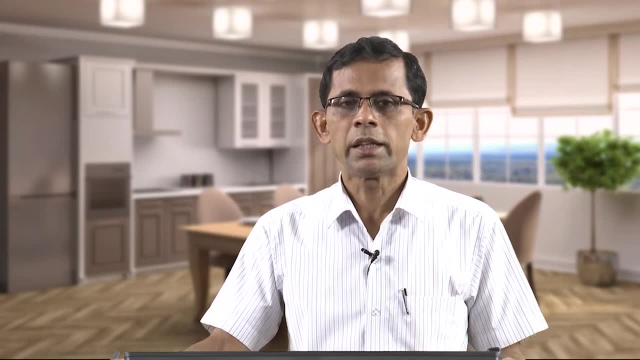 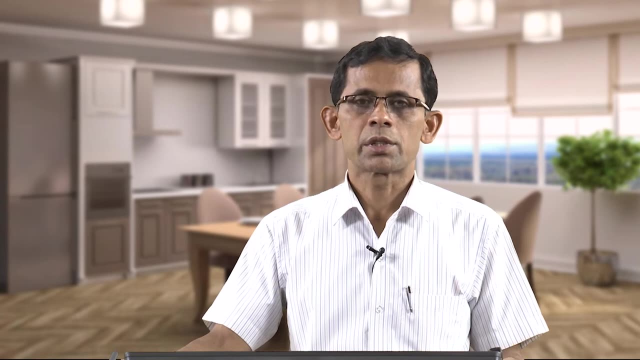 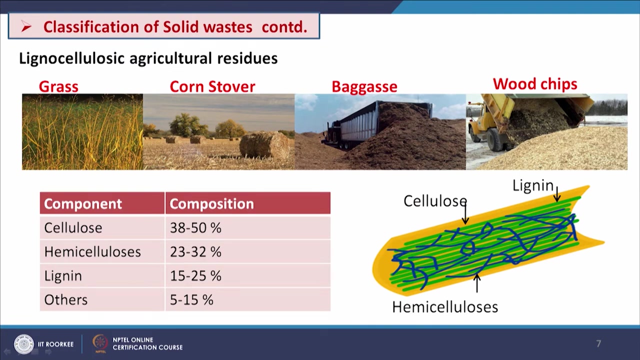 different. So the particular type of pollutants may be available in the solid waste and that has to be removed first before for the treatment using the conventional solid waste processes management processes. Now we will see the characteristics of the agricultural waste, that is, lignocellulologic biomass or lignocellulologic agricultural residues. So here some examples. 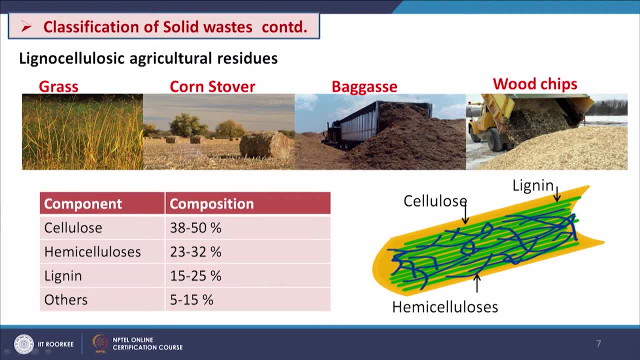 are given to grass corn stover by gas and wood chips, Thank you. And here we see cellulose, hemicellulose, lignin and others. component present in this type of materials is given in certain range. So suddenly we see that cellulose is present in the highest extent, followed by this hemicellulose. 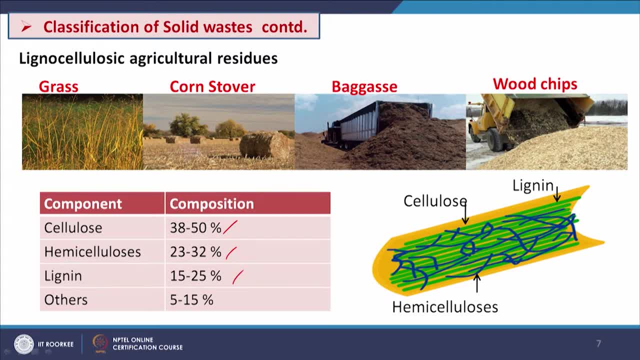 and lignin. And if we see that lignin, hemicellulose and cellulose have different structures, because all those compounds are having different chemical formula and their structure are different and some are having some crystal structure, like say cellulose and hemicellulose having 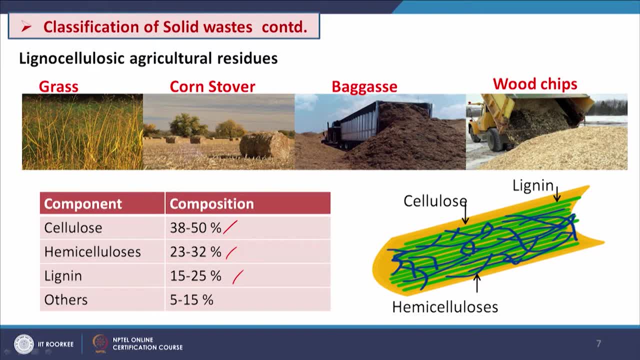 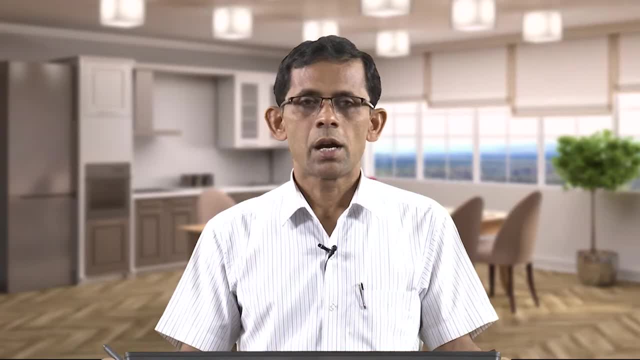 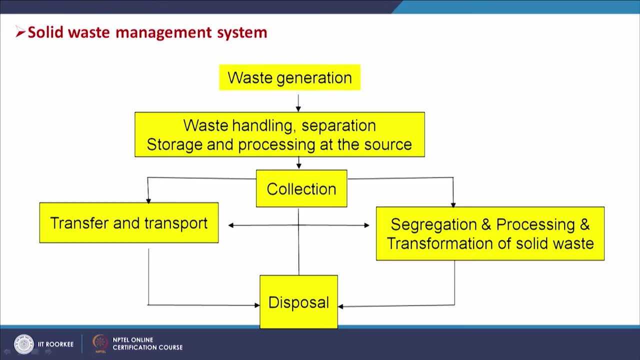 less organized crystals, and these are the structure of this. So this information will help us how to use this feedstocks or these wastes as a feedstock for the production of energy. Thank you. Now we will discuss the solid waste management systems. So now we have seen the different types of solid waste are generated, including MSW industrial. 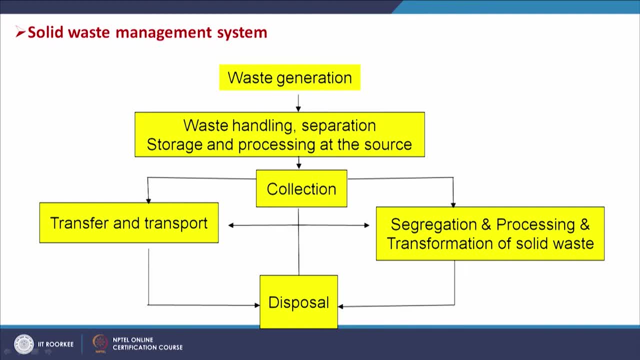 waste, agricultural waste, etcetera. Now our objective will be how to manage these wastes. particularly the management of MSW is a very big challenge, So it requires technological application as well as the management concepts or management application. So if we consider the management of solid waste, so first will be the source of generation. 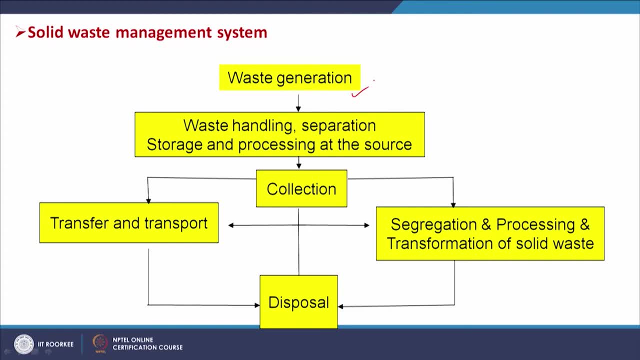 of the waste. So we should try our level waste to reduce less waste. So that will be the first principle or first philosophy for the solid waste management. Then when it is generated, then that has to be handled and collected properly. So waste handling, separation, storage and processing at the source. 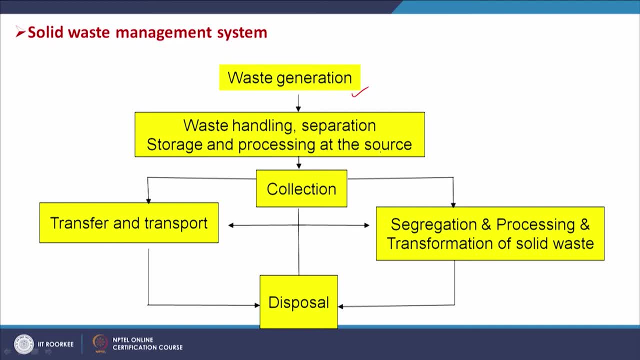 Each and every individual houses, we produce solid waste, So we should take care that we will producing less solid waste and once the solid waste which is generated, that has to be managed properly. It has to be, it has to be handled properly so that it will not create environmental hazards. 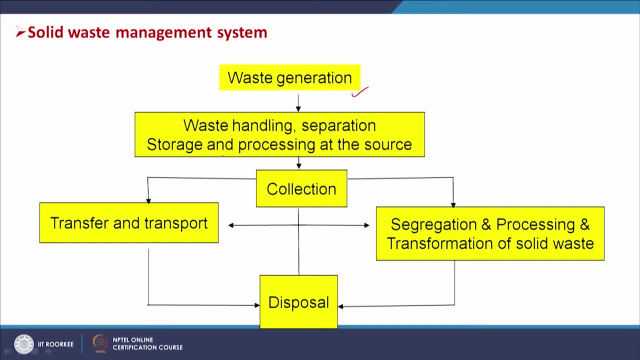 in the surroundings and that after this storage and processing at the source, at the source level And each individual houses, we can segregate the solid waste into different fractions and municipality can implement a methodology to collect different fractions for their proper management. And then collection system. is there that collection? there are different techniques. 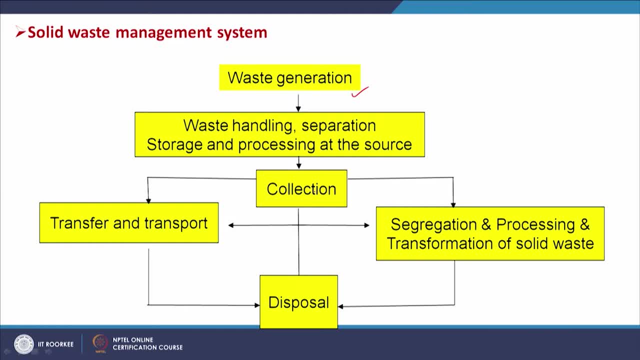 available for the collection of MSW from each and individual households and after this collection it has to be transferred and transport to the processing section or where the segregation and processing and transformation of solid waste are taking place. So after that, the segregation and processing, that means, as you have mentioned, there are 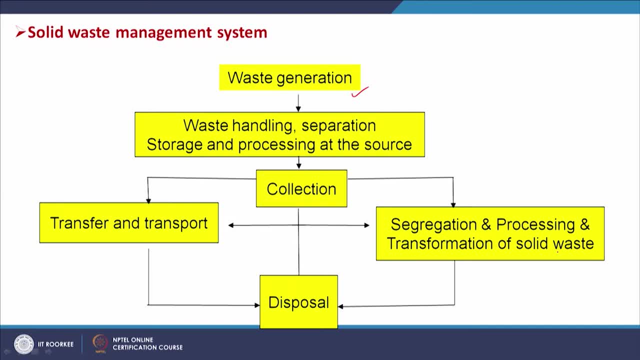 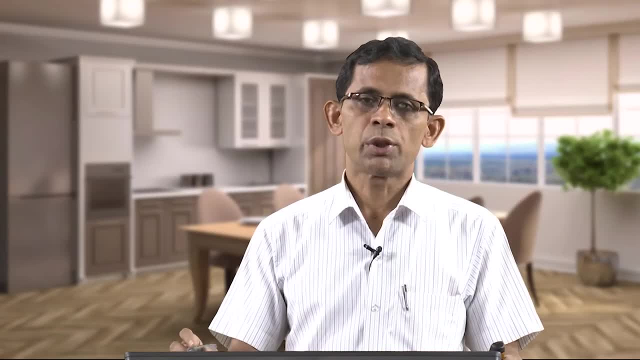 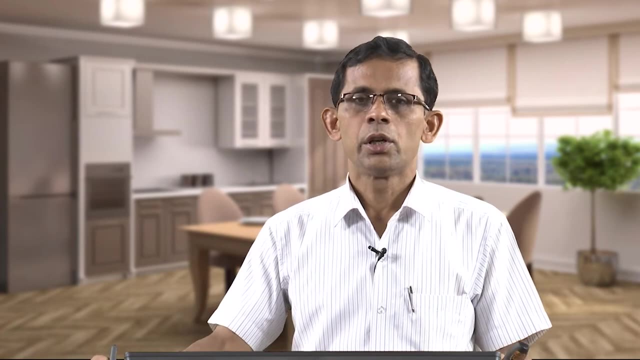 recyclables. there are organic compounds and there are inert. So, after this recyclable, after this segregations, we can. we can select particular routes for the processing of different fractions, For further utilization, value recovery, as well as to reduce the volume of the waste. 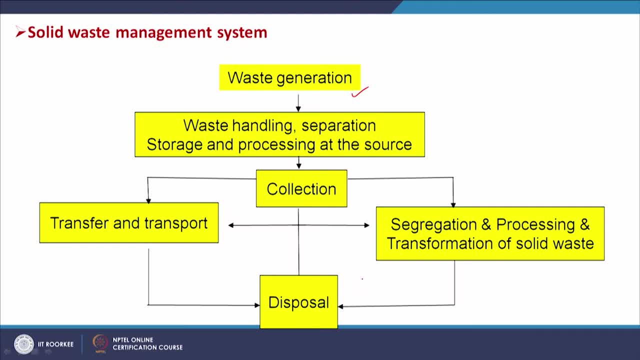 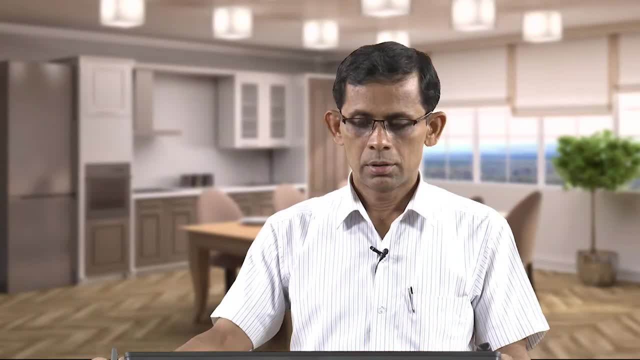 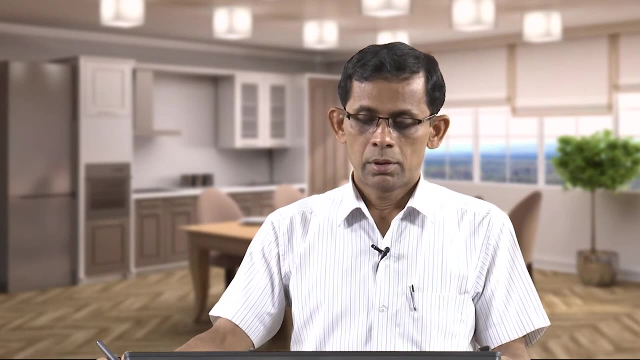 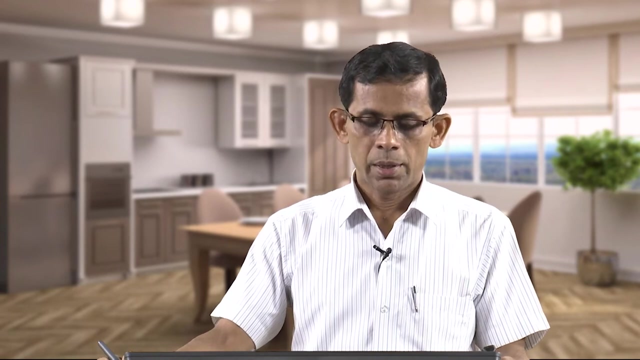 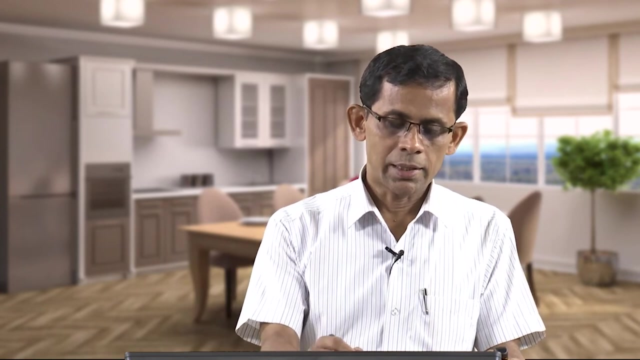 so that reduced volume will further be disposed. okay, So this is the scheme for the waste management, particularly the MSW, and so now we will discuss all these functional elements now. So waste generation: Waste generation and collection, So waste can be generated in a low building or high rise building, low rise and high rise. 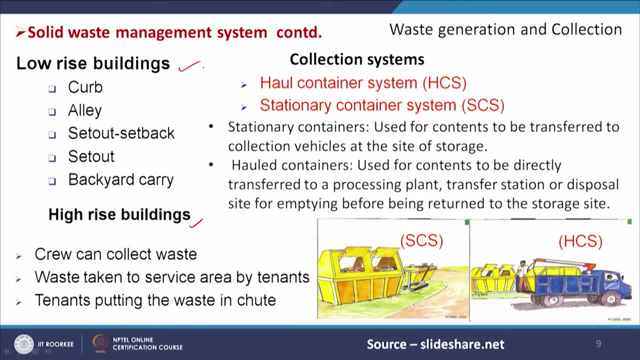 buildings. So for these two different types of buildings, different types of methods have been applied and implemented for the collection of the solid waste, Like say for high rise building, curve alley set out, set back, set out, backyard carry. 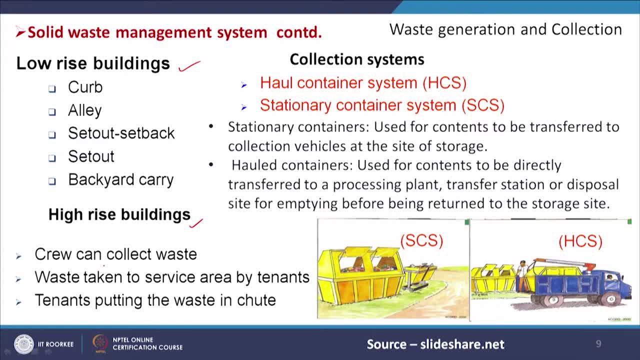 all those things are there And high rise building screw can collect waste, waste taken to service area by tenants and tenants putting the waste in tube. So these are some methods which are used in different part of the world for the collection of the solid waste. 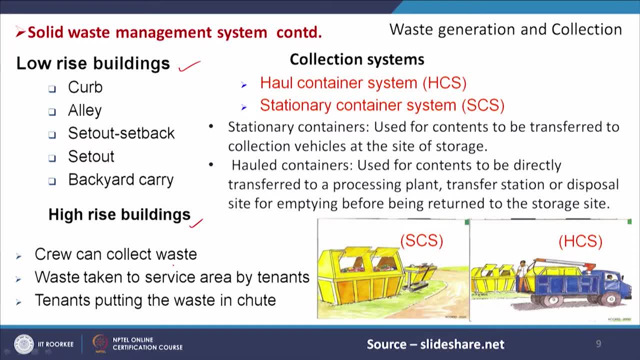 And if we think about the collection systems, so basically major two types of collection systems are used. One is your haul container systems and another is your stationary container system. So stationary container systems, So stationary container systems- are basically used for contents to be transferred to the 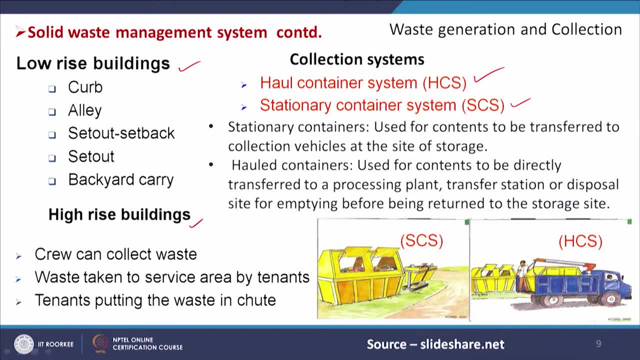 collection vehicles at the site of storage. So this is the site of storage. Waste are collected here. So transport or municipal vehicle will come, So here this waste will be transferred. So that is your stationary container system, But in case of haul container system this is used for the contents to be directly transferred. 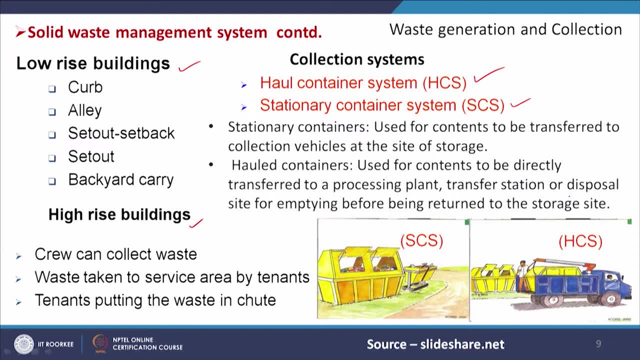 to processing plant, Transfer station or disposal site for empty container. So that is the collection system. But when the container is empty it will be returned to storage site. So the container is taken to disposal site and the processing site with the carrier. 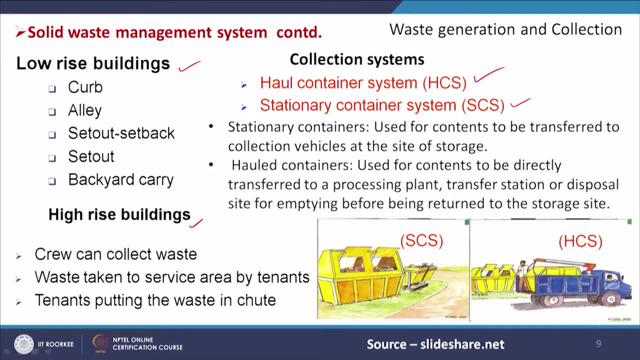 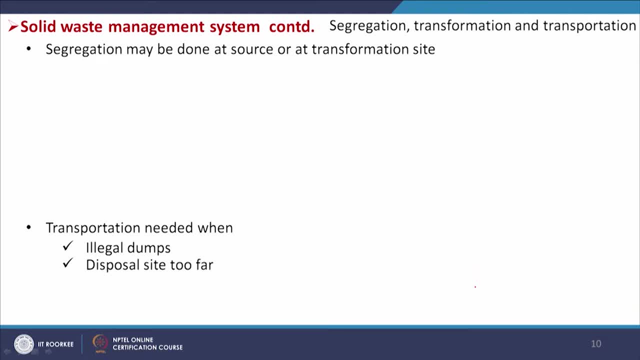 And then, after unloading, it is again returned to this place. So that is the haul container system. So these are the different types of systems which are used for the collection of the solid waste- municipal solid waste. So these are different types of systems used for the collection of municipal solid waste. 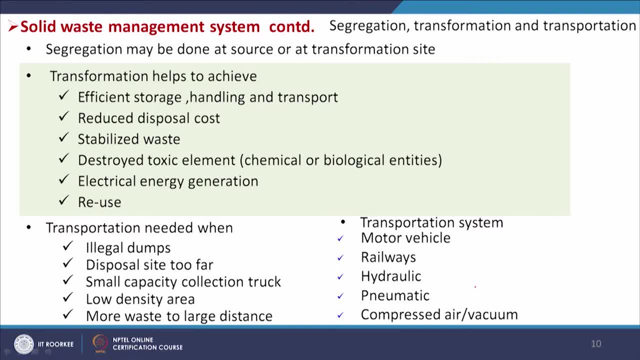 in different parts of the country and in the world. So this is the collection system. Now we will see the segregation, transportation, transformation, segregation, transformation and transportation. So segregation may be done at source or at transportation site. so when it is transformation site, so when we are going to transform it, that means we 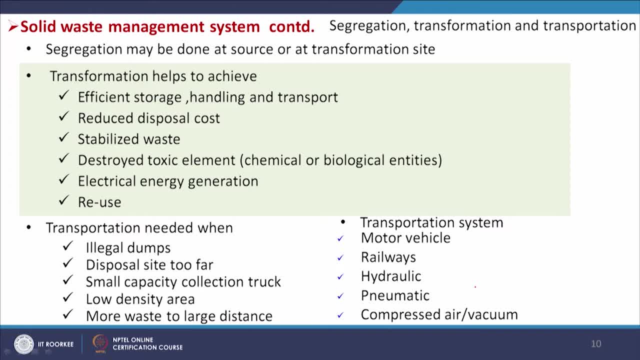 are going to extract energy or some other valuable from it, so at that site, or it can be sorted at the site where it is being generated as well. So transformation means you know the value, addition or extraction of energy and other products and reduce the volume of the residue, basically, and this transformation helps to. 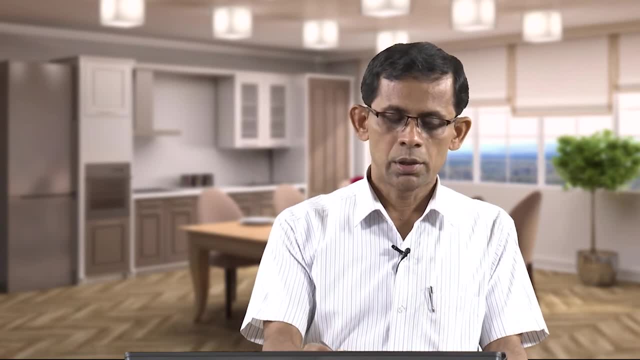 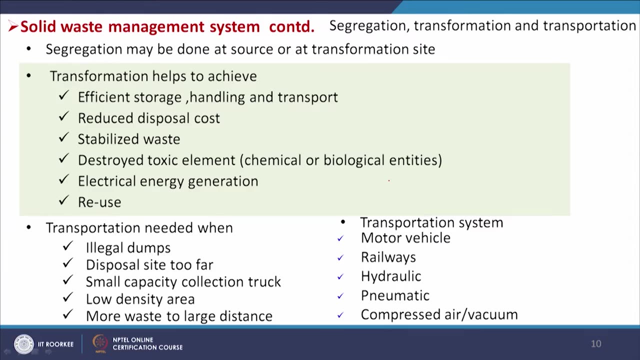 achieve efficient storage, handling and transport. reduced disposal cost, stabilized waste, destroyed toxic element, that is, chemical and biological entities, those are being destroyed, electrical energy generation and reuse. So these are the advantage of the transformation and transformation process. So transportation needed and the illegal dumps we want to prevent and then disposal. 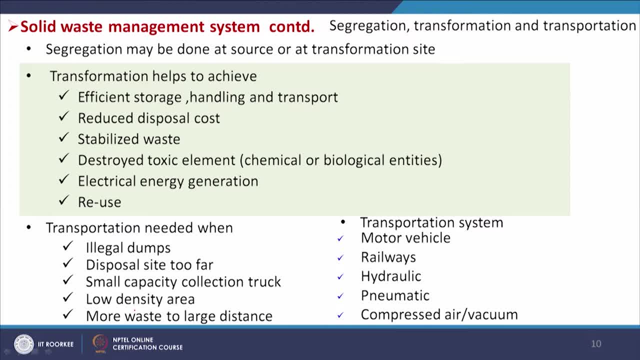 site too far and small capacity collection truck and low density area and more waste to large distance. So we have a certain area where the waste will be collected and disposed and then at that time this will be for away from the main city. so that is the reason. 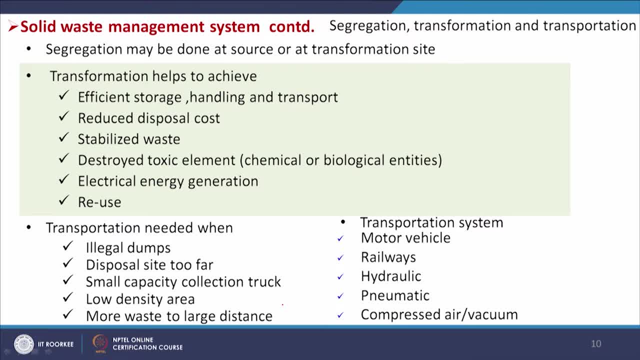 why this transportation is required and transportation. different types of transportation should be used. So the transportation of the waste can be used like motor vehicle, railways, hydraulic systems, pneumatic conveying systems and compressed air or vacuum. So these are depending upon the situation. in our country, mostly motor vehicles are used. Now we will see the disposal. options. So disposal of wastes: the residual part of the solid waste after transformation which is remaining that has to be disposed. So disposal of waste: the residual part of the solid waste after transformation which is remaining that has to be disposed. And there are many methods through which the disposal can take place: Open dumping land. 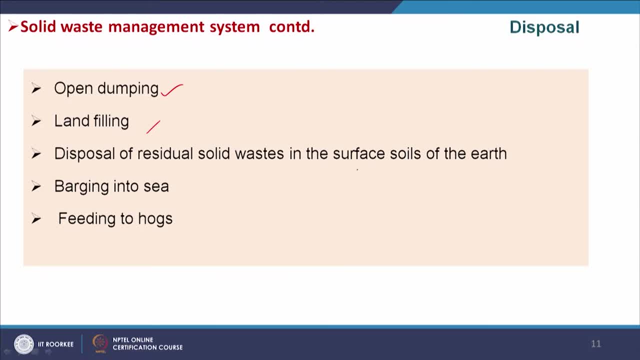 filling, disposal of residual solid waste in surface soils of the earth and burying into sea and feeding to hogs. so these are some generally used disposal methods. We will discuss the land filling and others also. So open dumping we have seen it is open it. 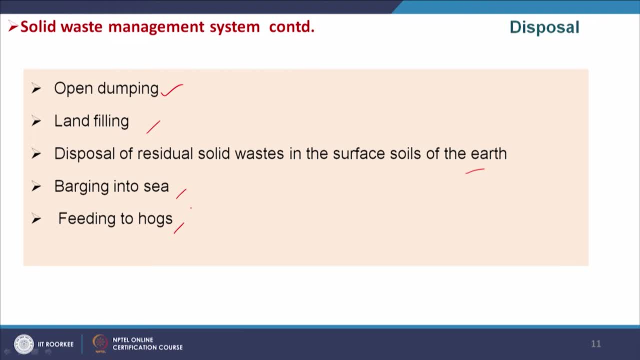 it is practiced in most of the towns and cities in our country And land filling is also implemented in metro cities and some other cities in the country And burgeoning into sea. that was a good option once, but now a days it is not encouraged. 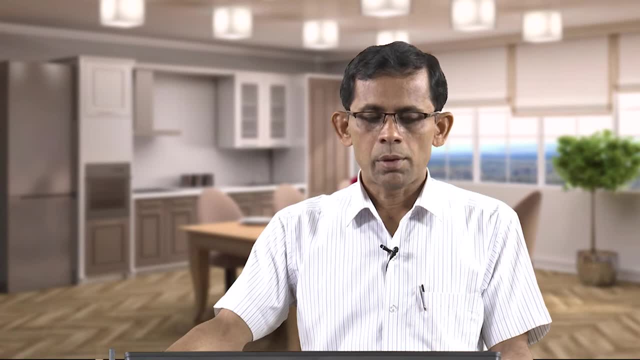 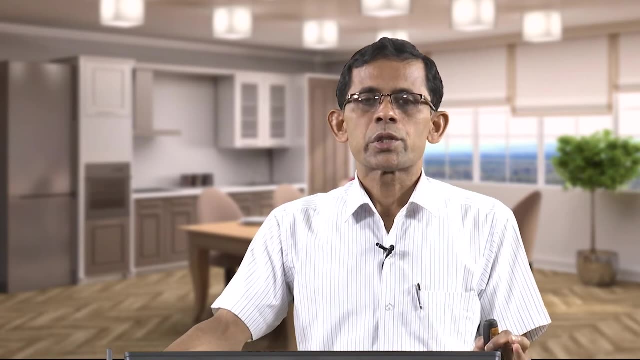 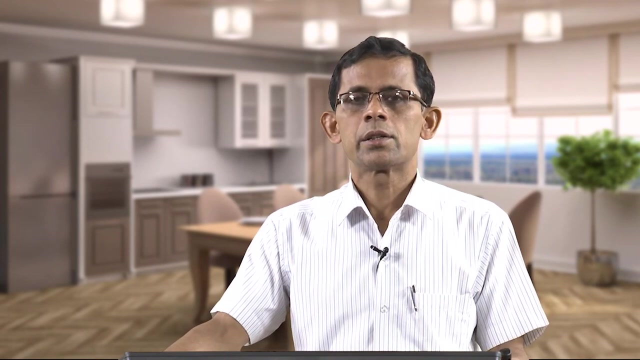 Now we will see the roots of solid waste management. So those are the disposal option we have seen. We have seen that waste, solid waste or MSW, has to be collected, it has to be segregated, then transformation and then residual will be disposed of. So these are the basic steps. 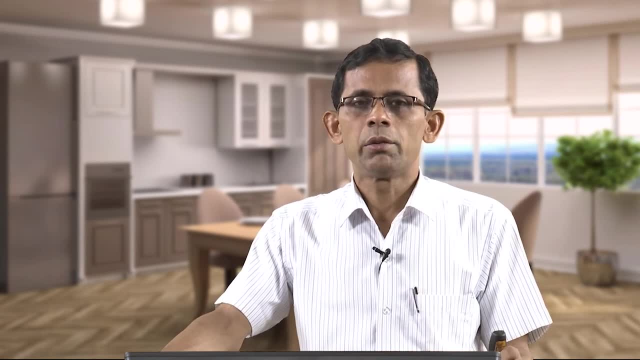 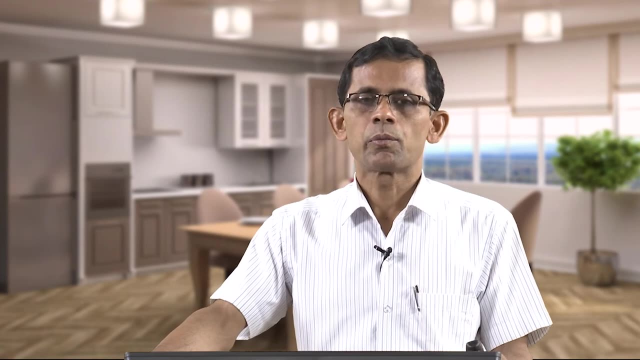 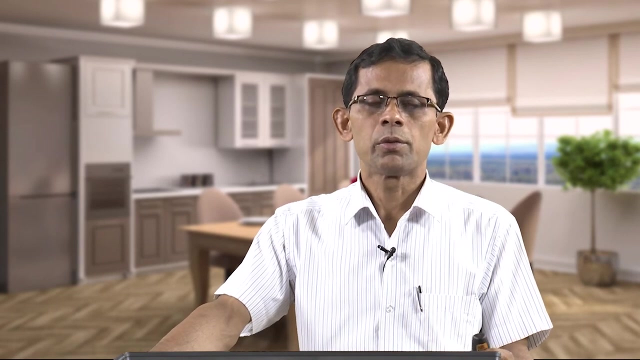 Now we have also seen that MSW, or solid waste, may be of different types, Like, say: someone is recyclable, some part is non-recyclable, some part will be having organic content, some part will not be containing any organic, or some part it will be containing. 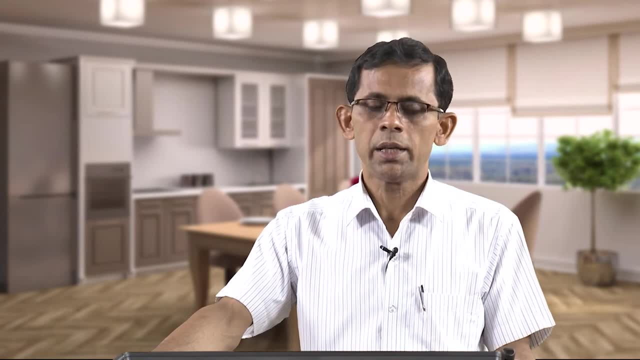 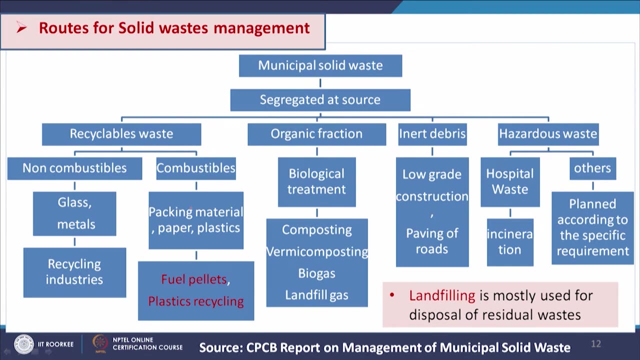 more moisture, some part will be containing less moisture. So likewise we will see different type of wastes, how we can manage it, So segregated at source. the first step is to segregate. Second is to identify different fractions like, say, recyclable, Recyclable waste and then organic fraction, inert debris and hazardous waste. 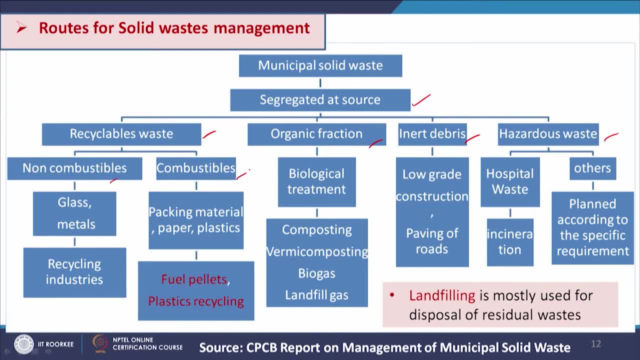 So if it is a recyclable waste that may be non-combustible or may be combustibles- If it is non-combustible, like, say, glass, metals etc. So those will be used in the industries through the recycling process, And if it is a combustible, then those can be used for the 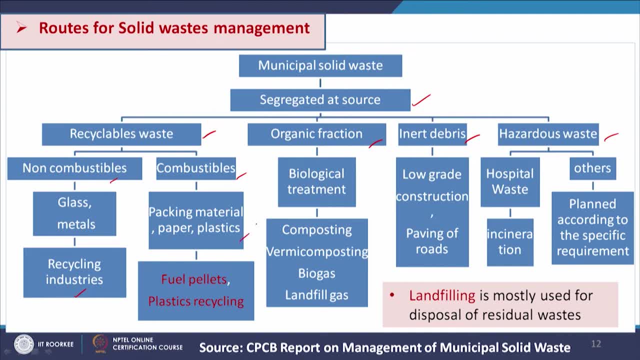 energy production and like, say, packaging material, paper, plastics- these are some examples. So those can be used for the recycling- Fuel pellets productions, and the plastics can also be recycled to produce different types of products. So this is one way of the management of the recyclable wastes. 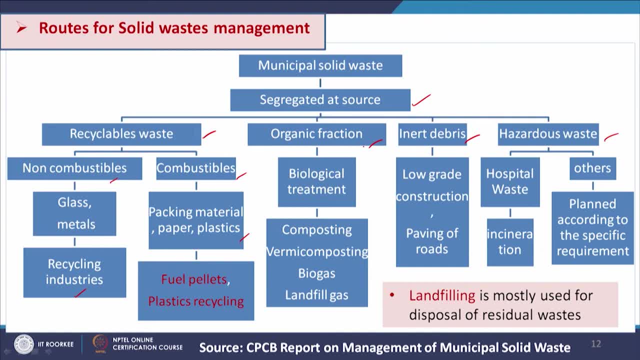 And then some other type of materials which is having organic fractions- high organic fractions, like, say, biological treatment can be suitable for that, And composting, vermicomposting, biogas and landfill gas production can take place from this type of solid waste Already. 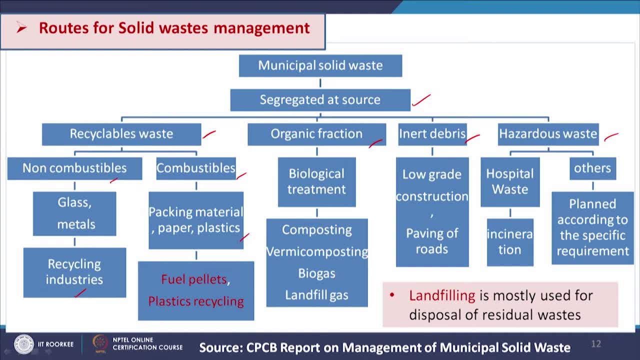 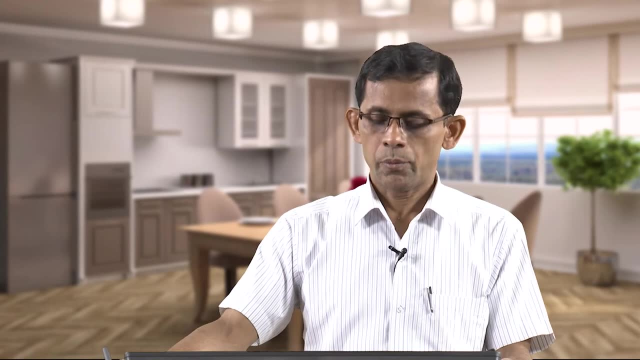 we have discussed About the composting, vermicomposting and biogas production, and landfill gas is produced in the similar way. Similar types of reactions are also responsible for the production of landfill gas, like anaerobic digestion, So we will discuss this one. And for inert debris? 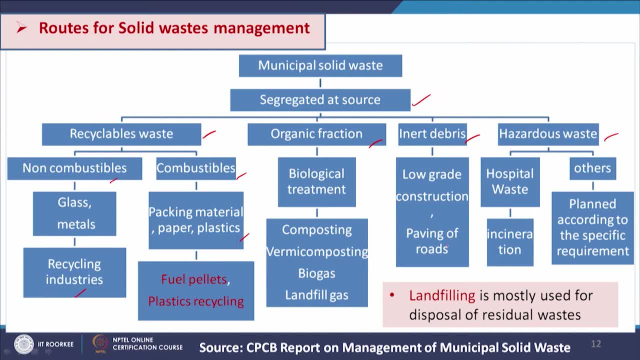 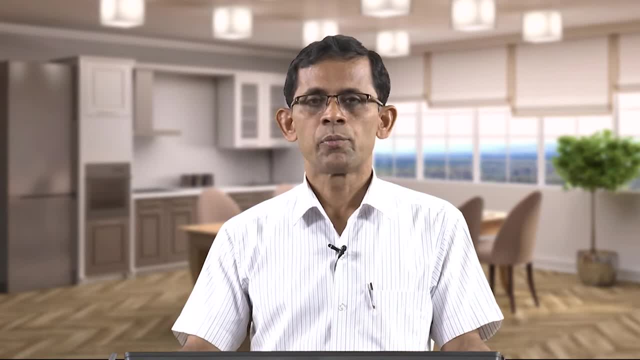 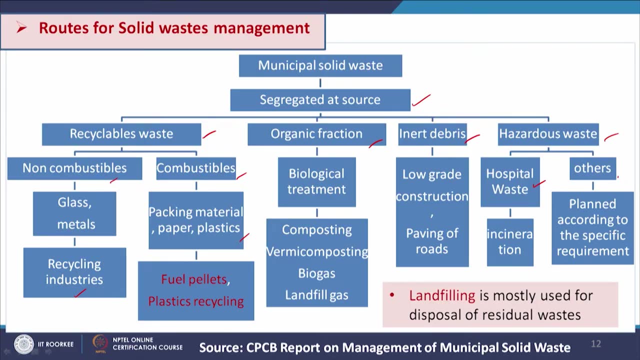 those are not having any carbon content and those are not suitable for energy productions or valuable extractions. So those will be used, or those can be used, for the road constructions or paper productions or paving of roads, And if the material is of hazardous in nature. 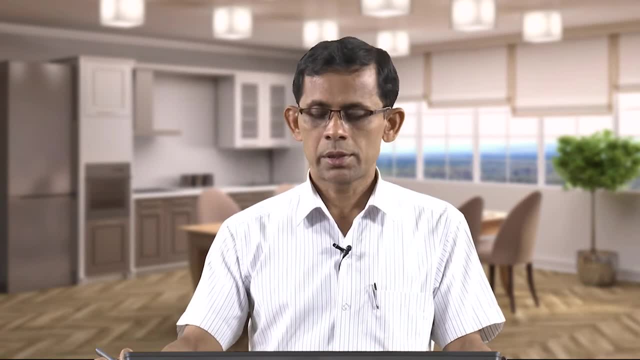 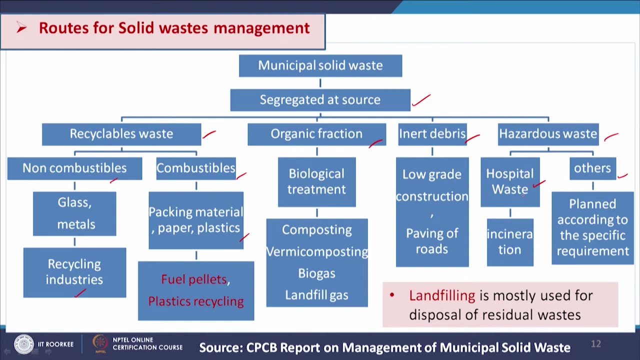 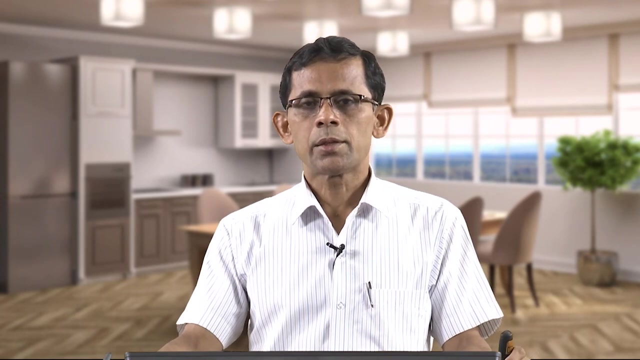 then that may be of from different sources, may be from hospital waste or may be from other sources. In the solid waste which comes from hospital waste, all are not having the hazardous characteristics. Some of those are having hazardous characteristics So they will be used to make the process. 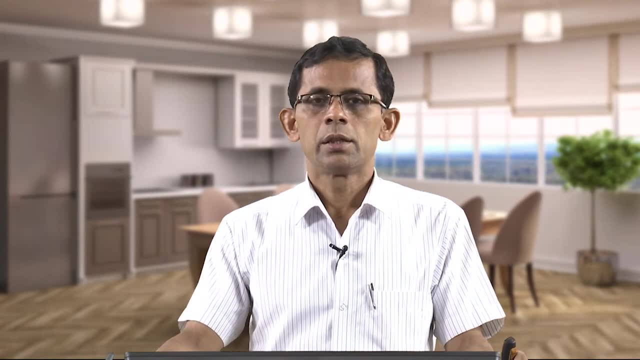 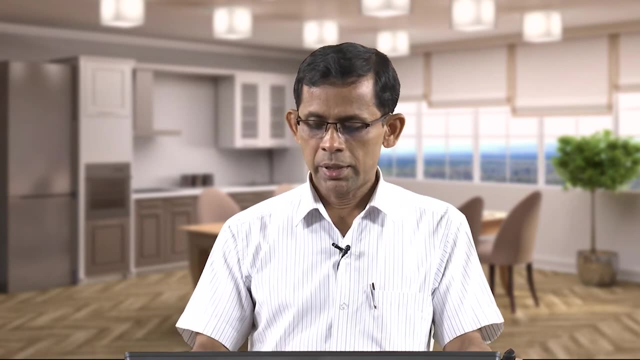 So we have discussed these aspects And then we have to discuss now that how the waste is used in the construction process. So this is classified as a special category waste and we will discuss it in detail for its management. And one example is given here: that incineration. that is one of the method. 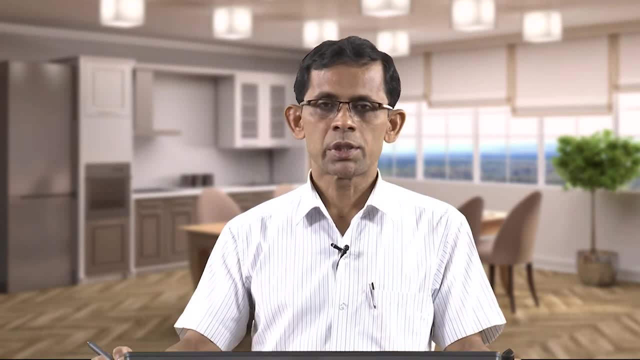 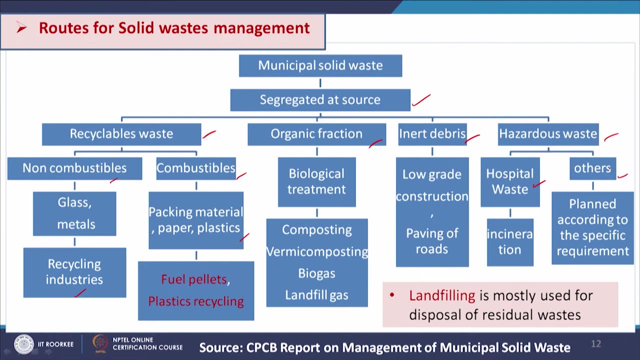 which can be used for managing this type of waste- but we will be having more discussion on this in detail- And some other type of wastes maybe, like, say, e-waste or any other type of waste, So those are may be a special type of waste, So this is classified as a. 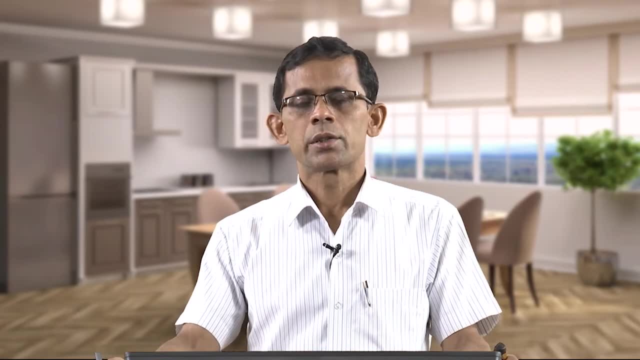 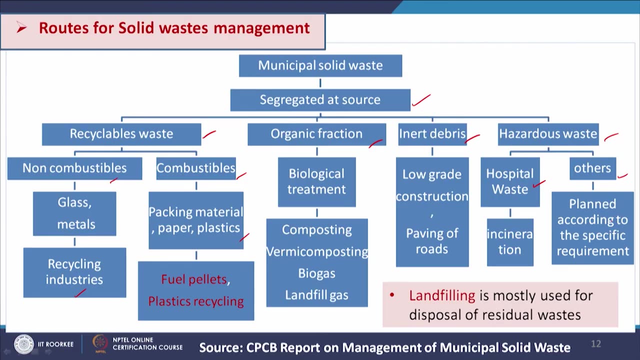 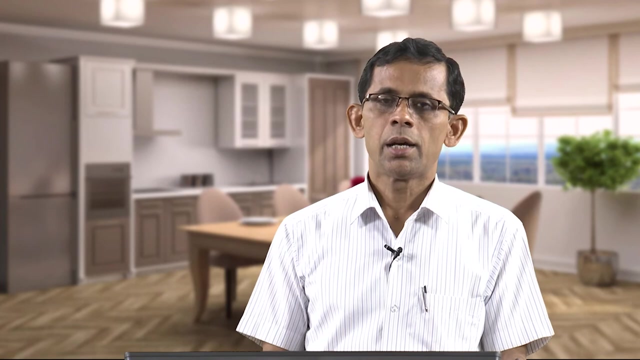 waste. So for those waste materials, some special methods are recommended and those are followed. So, accordingly, the plant according to the specific requirement, So management can be planned according to the specific requirement, and whatever may be the residual part generated from different methods that can be ultimately disposed through landfilling, So landfilling. 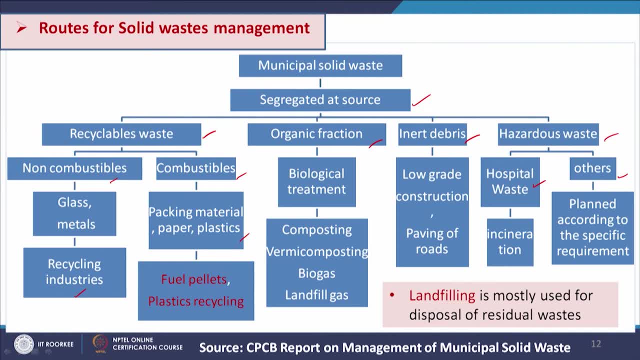 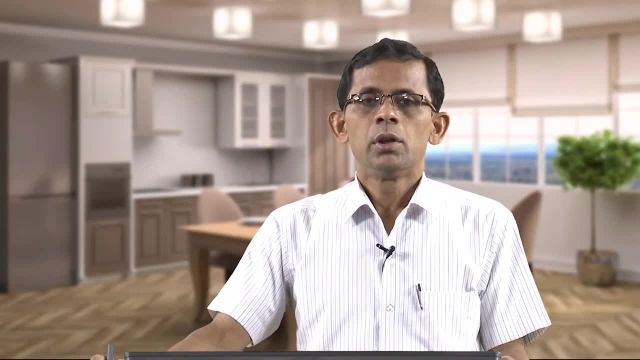 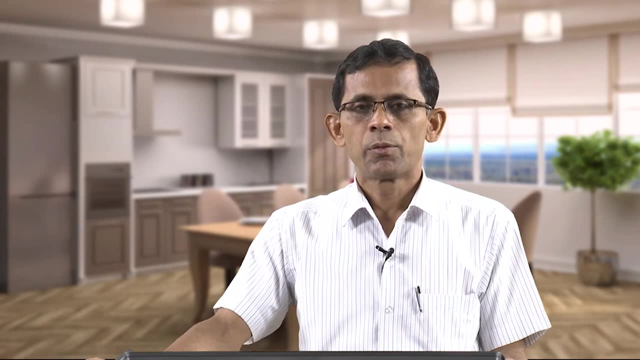 is the mostly used for disposal of residual wastes. So this is the routes or schemes for the solid waste management. Now we have come to know that some part of the MSW which is having high carbon and hydrogen content and heating value, those can be converted. 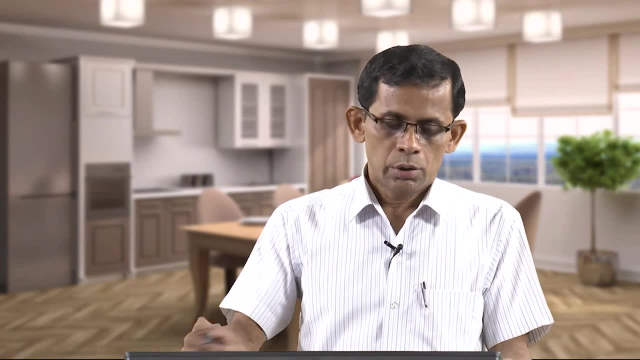 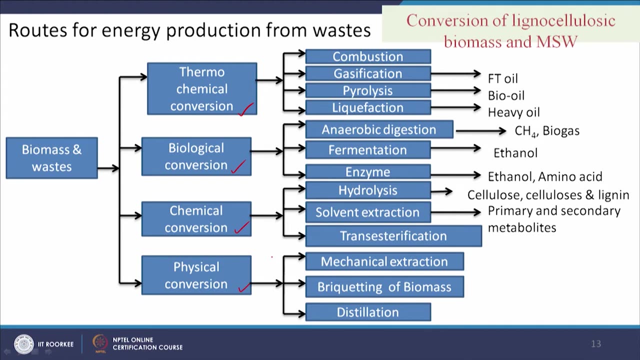 to energy, So that conversion can take place basically through thermo chemical conversion, biological conversion, chemical conversion and physical conversion. And physical conversion like say, mechanical extractions, briqueting of biomass and distillation. So these are the prerequisite for some other type of conversions and thermo chemical conversions like combustion. 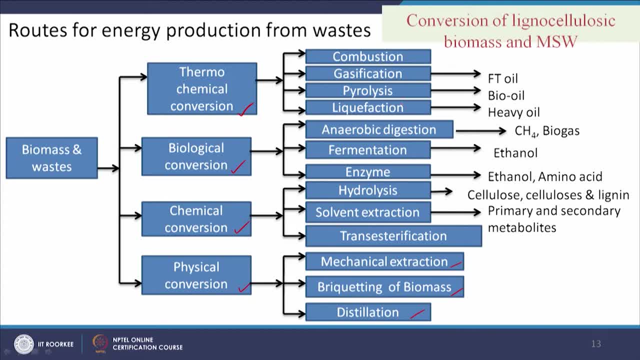 gasification, pyrolysis, liquefaction, which are very important, and those processes give us different products like FT oil to gasification, bio oil from pyrolysis, heavy oil from liquefaction and biological conversions And anaerobic digestion, fermentations and enzymatic reactions. So that can gives, say, 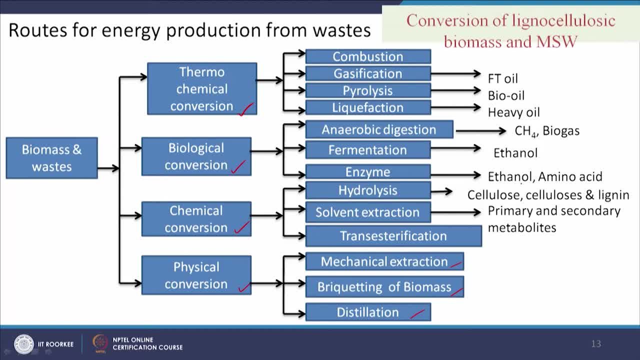 methane or biogas, from fermentation ethanol, and from enzymes, ethanol, amino acids, etcetera, And chemical conversion like hydrolysis, solvent extractions and transesterification methods are used. So here cellulose, hemicellulose and lignin. through this we can get ligno cellulosic. 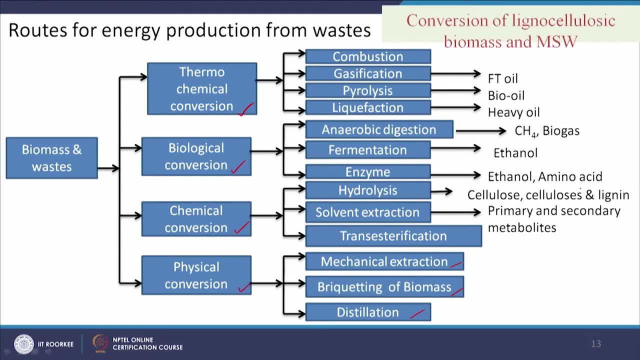 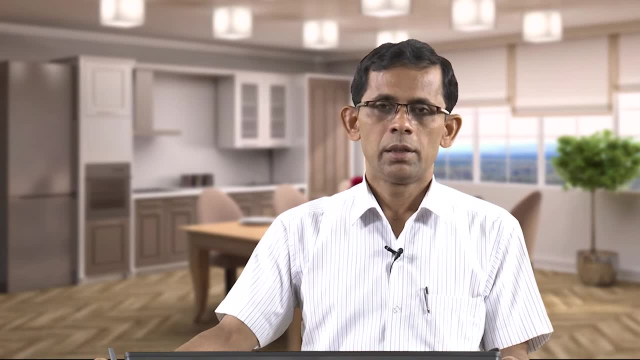 materials to cellulose, hemicellulose and lignin, And then solvent extraction give us primary and secondary metabolites. So these are the different methods which are used for the transformation of the solid waste for energy production. Now we will see what is landfill and we will discuss on. 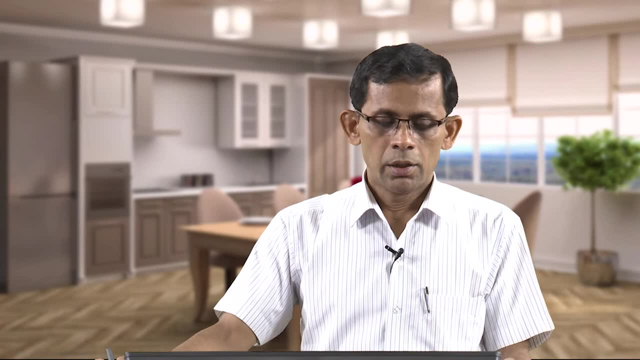 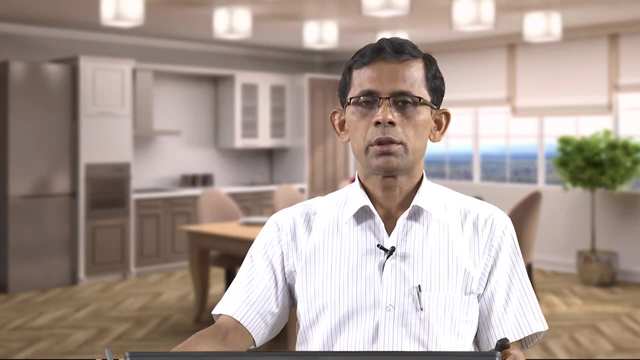 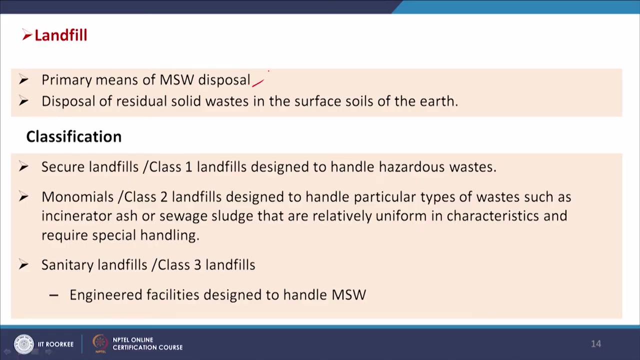 it. Now we will discuss on landfill. So we have seen that landfill is one of the important method for the final disposal of the residual So that it primary means of MSW disposal. we can say We can say it is the primary means of MSW disposal And disposal of residual. 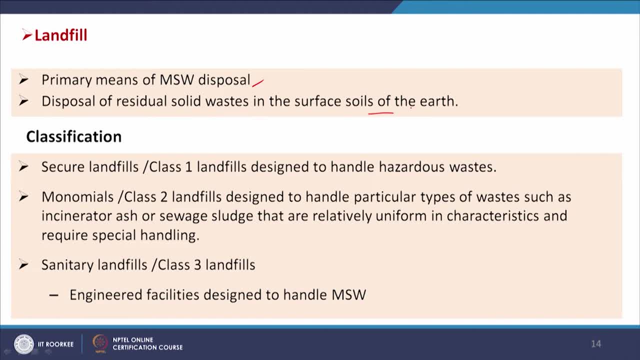 solids in the surface soils of the earth. How it is done We will see in the surface soil of the earth And then, depending upon the nature of the solid waste the land fills, maybe of different types or may be classified into different category, like, say, secure landfills. 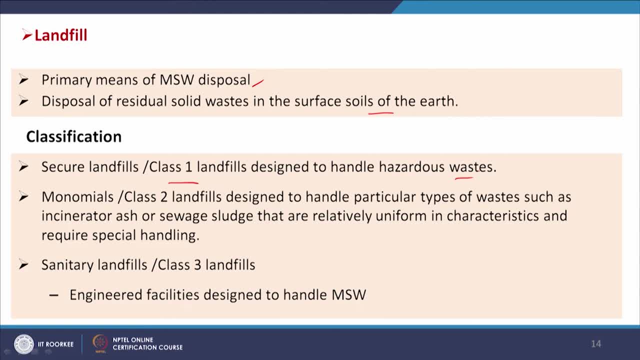 class 1 landfills that is designed to handle hazardous waste, And then monomials are class 2 landfills designed to handle particular types of waste, such as incinerator ash and sewage sludge, that are relatively uniform in characteristics and require special handling. 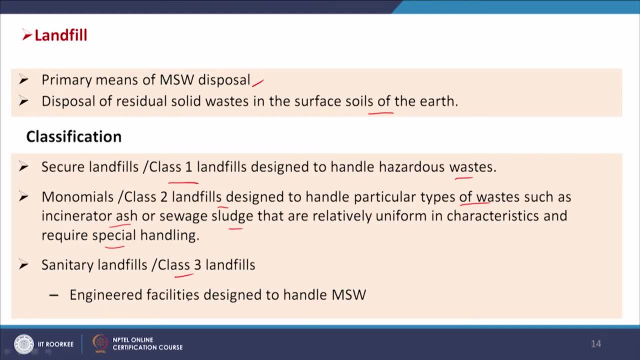 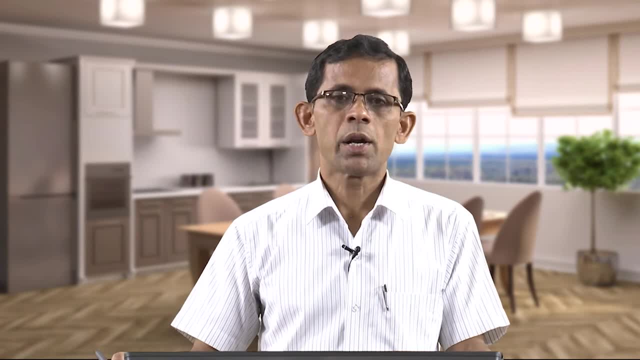 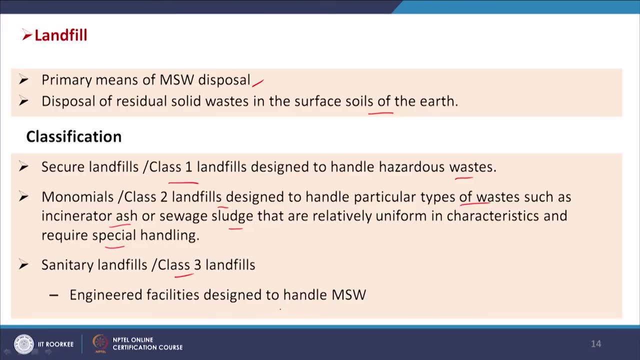 And sanitary landfills, that is, class 3 landfills that basically is suitable for non-hazardous materials and the residual part of municipal solid waste are processed through this route And engineered facilities are designed to handle MSW. so these are the different types. 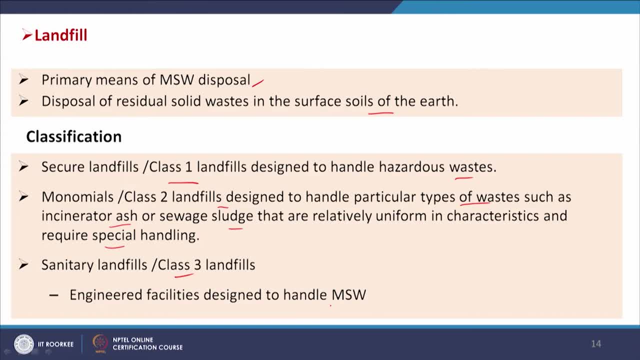 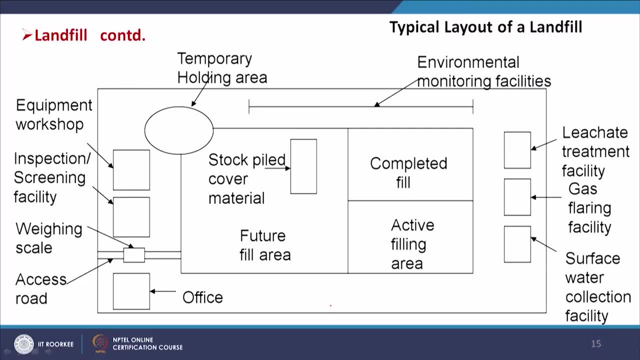 of landfilling sites, which are used for the handling of the residue of different types of solid waste. If we consider a landfilling site, so you will see that there are some active filling area. So the residual part of the MSW is coming and dumping here, and then this is lowland. 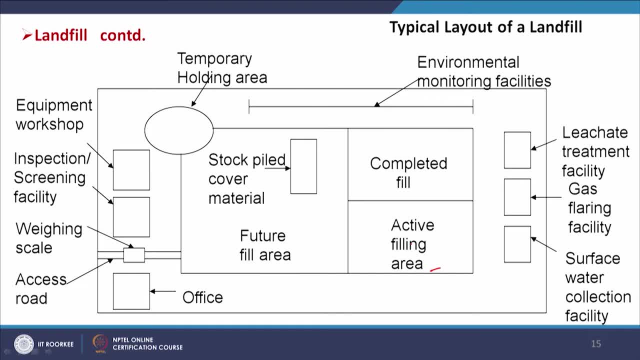 and then there will be some soil cover for everyday filling. there will be some soil cover and when it will be complete- then they complete- it will be covered with sand with certain thickness And then this will be filled and next there will be some area for future fill area and 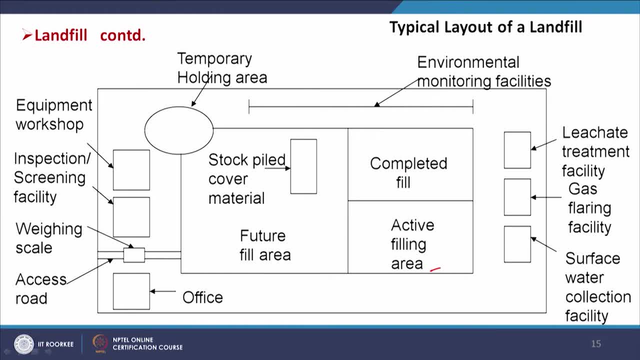 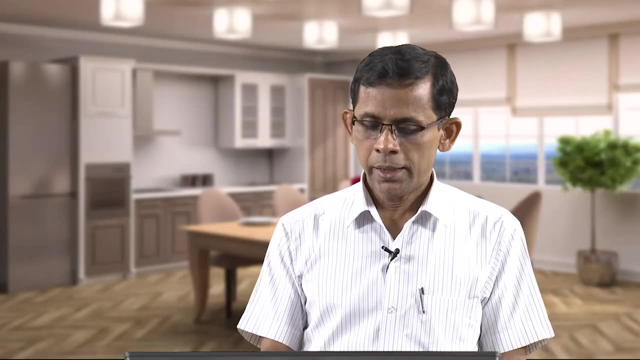 certainly there are some area where already the land field has been completed. So completed field and then active filling area and future area. those are very, very essential area requirement for the land filling. We also put some soil every day, So stockpiled for cover material is also needed. 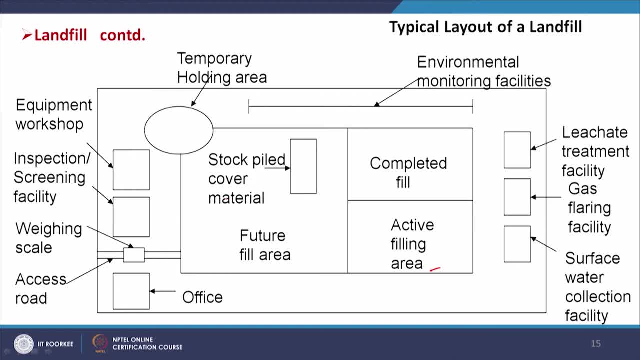 We need to store somewhere. So these are the different area requirement for the operations of the land filling. Apart from this, we have discussed that this land filling will be creating some leachates and there will be some landfill gas production. So there will be some leachate treatment facility, gas filling facility and surface water collection. 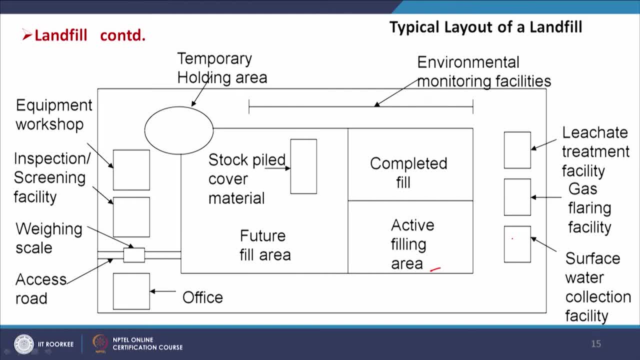 facility. So these are very essential part of a land filling area And we also need to manage the environmental qualities. So environmental monitoring facilities are required and temporary holding area is also required And it also need one office space and road for access and weighing scale inspection. 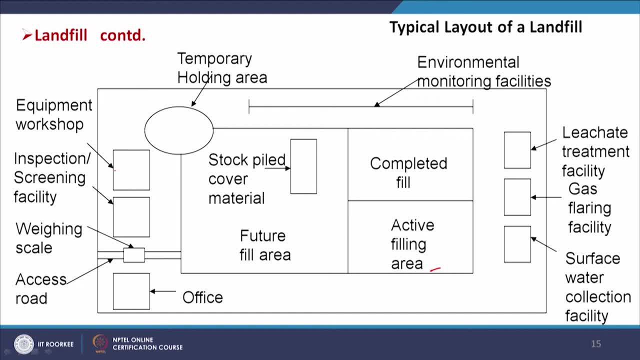 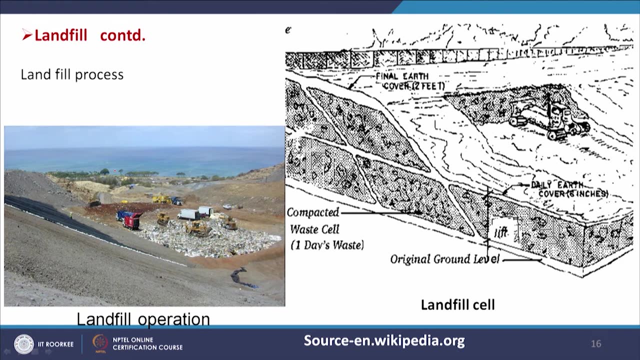 and screening facility and equipment or workshop. So these are the different parts of the land fill area. or we can say this is the typical layout of a land fill And if we see the land fill process, so here, land fill process, you see The residual material is collected and then it is put in the low land and it will be covered. 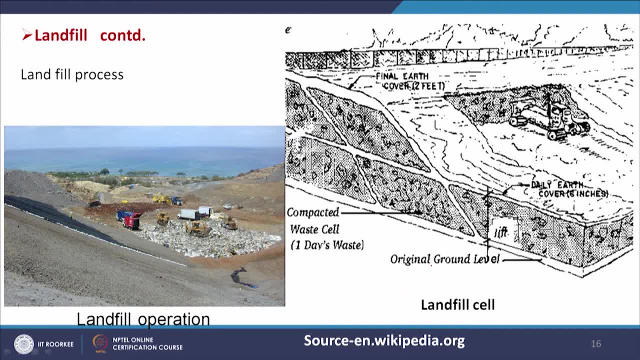 with the soil As shown here. this is original ground level. So this is compacted waste cell. Waste material is compacted. here You see some rollers are running, So it is being compacted. And then daily earth cover. So you see some rollers are running. 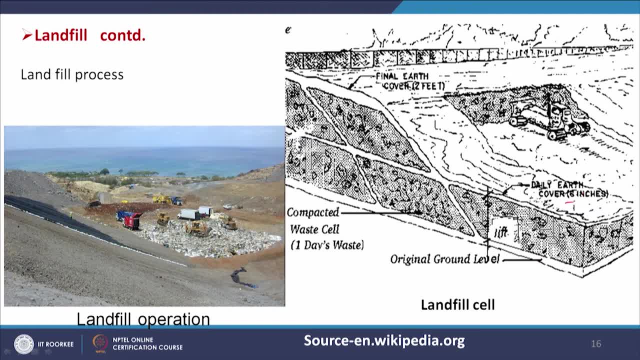 So it is being compacted And then daily earth cover, So 6 inch cover is there After one day compaction. some earth is given on the solid waste, Then solid waste residue, some earth material is given, And then it is covered. 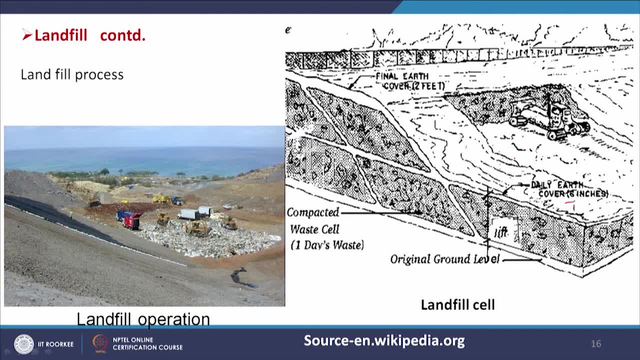 And then it is pressed and compressed And then daily we will having the same operation and the daily basis. we will be having the same type of filling and daily basis, And when the complete fill will take place, then ultimately, final earth cover of 2 feet. 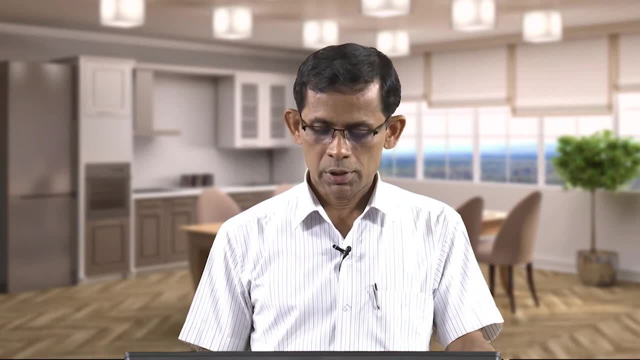 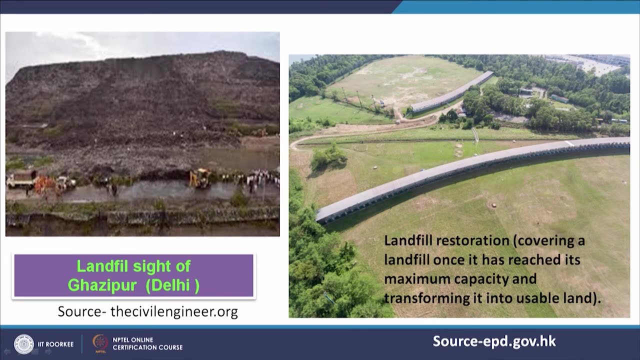 has to be provided at the top. So this is the fill process and this slide shows us some live photographs of landfill sites at Ghazipur, Delhi, and this shows us the. this is your active sites and this is your filled site, where the land filling has been done and that area is restored. 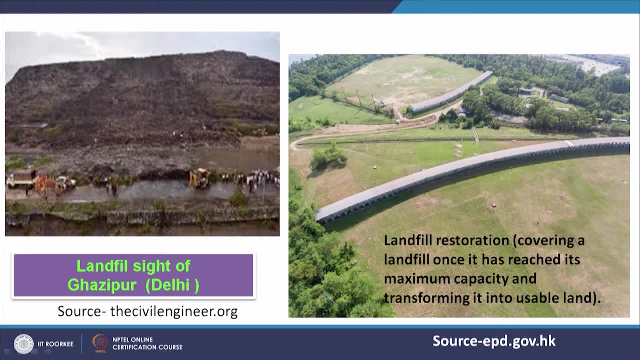 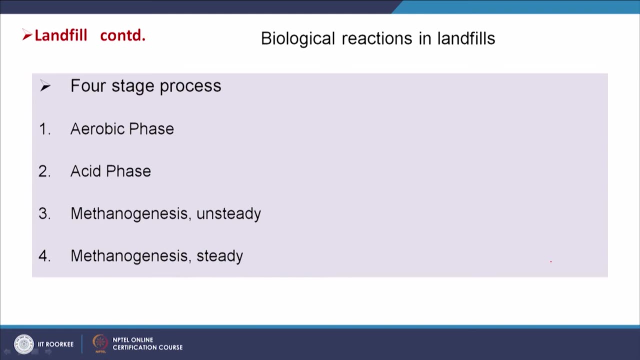 So landfill restoration, that is, covering a landfill once it has reached its maximum capacity and transforming it into usable land. So this is the example of the restoration of the landfill and different types of reactions which can take place in the landfills, that those are similar to anaerobic digestion reactions. 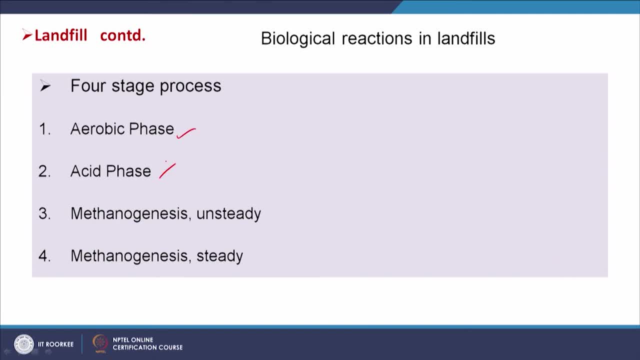 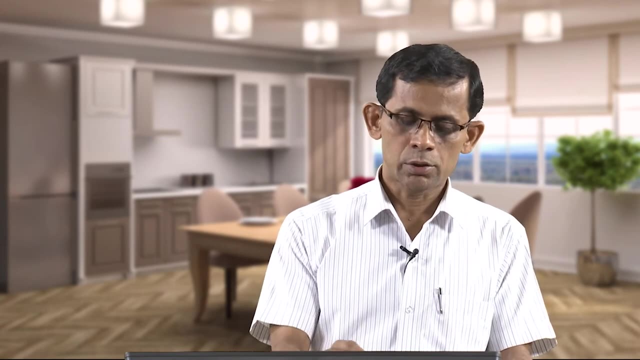 like, say, aerobic phase and acidic phase and then methanogenesis and methanogenic phase. So in this case, at the top part there is the possibility of oxygen. so aerobic reaction can also take place. and as we go inside, when the depth increases, then acidic phase reacts. 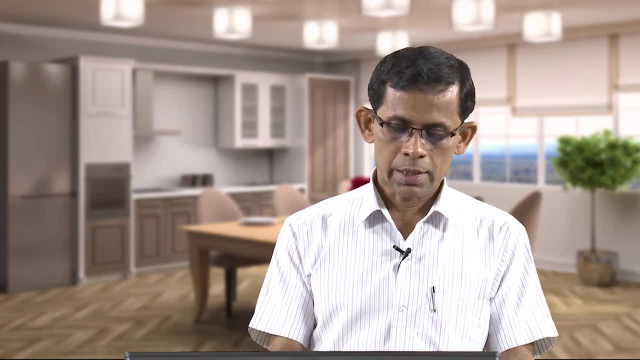 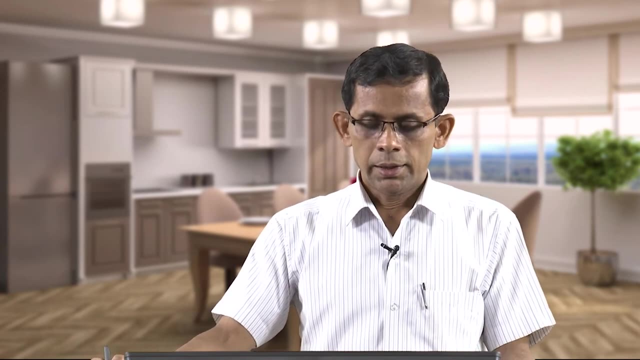 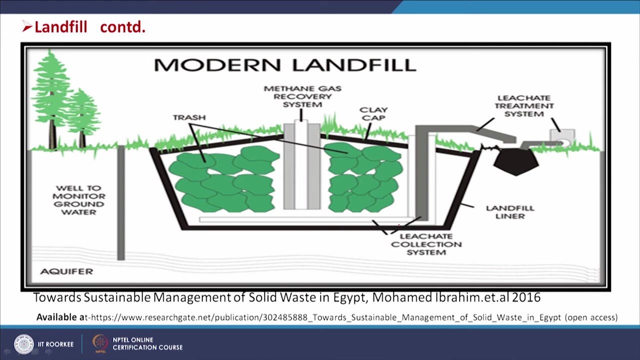 then, after acidic phase, methanogenesis reaction takes place. this is unsteady and then steady state. So similar reactions which take place in anaerobic digestion. and this is a modern landfill. so here we see. So this is your lining is done so for leachate collection and landfill liner is shown here. 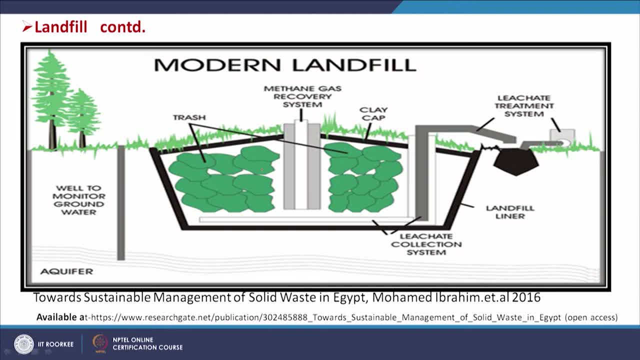 and this leachate treatment system is there and trash and clay cap is provided. at the top clay cap is provided and inside the trash the material is put here and methane gas recovery system is also there, so where biogas is produced and water is going there. 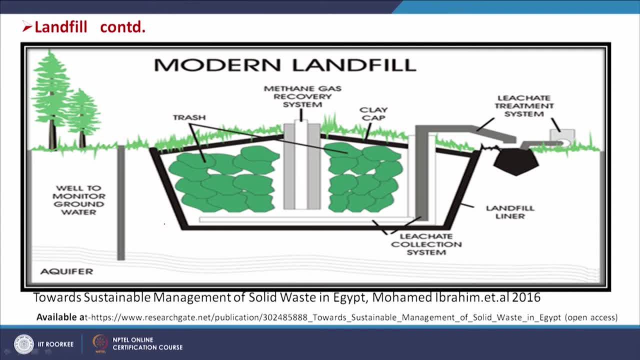 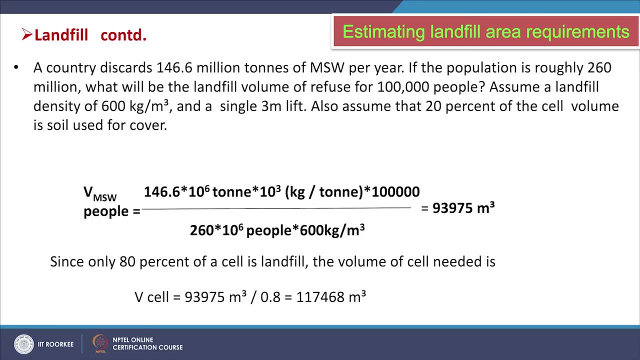 So, but this is not First of all if you look at the side label. So the bottom line is: adjustments were done. a vos is measured between the jeszcze u Penn. For what? 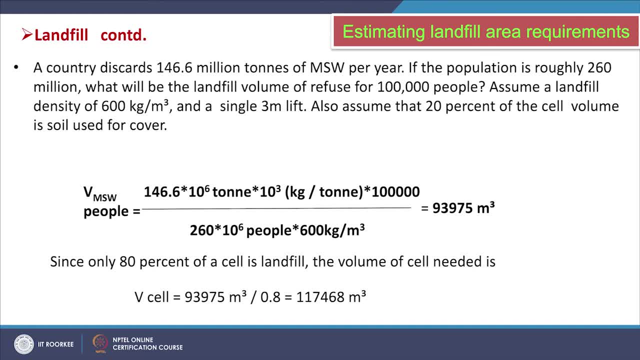 and a single 3 meter lift. also assume that 20 percent of the shell volume is well used for cover. So now we will calculate the volume of the MSW. So how can you calculate? We have total 146.6 million tons of MSW per year. So this into 10 to the power, 3 kg per year. 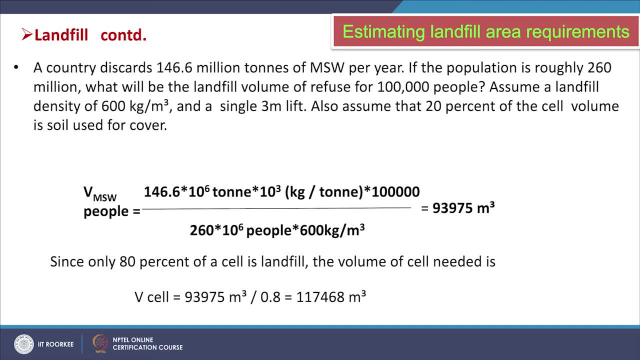 so conversion of ton to kg, and then we have this: 1 lakhs people, and for one lakh's people you have to calculate. So this waste is generated from 260 million people, so per unit people. So these divided by 6 into 600, because 600 is the density of the of the landfill. So 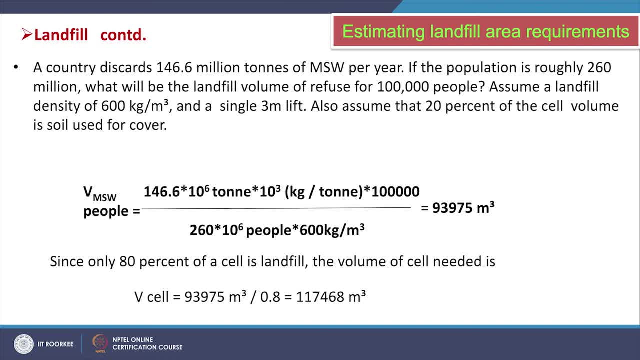 this is, We are multiplying this term and dividing it, this term, then multiplying this total people, So this will be the total mass of the waste generation, then divided by this density, so it is giving us the volume. So this will be the total volume, but 20 percent of the 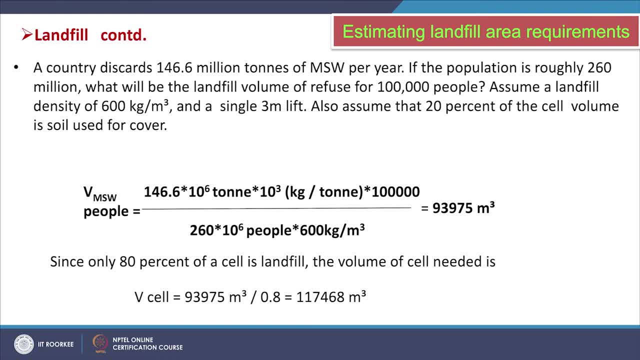 shell volume is soil, so that the actual volume will be more than this. So that will be divided by 0.8, so that is equal to 117468 meter cube. Now the area of lift at 3 meter shell depth. 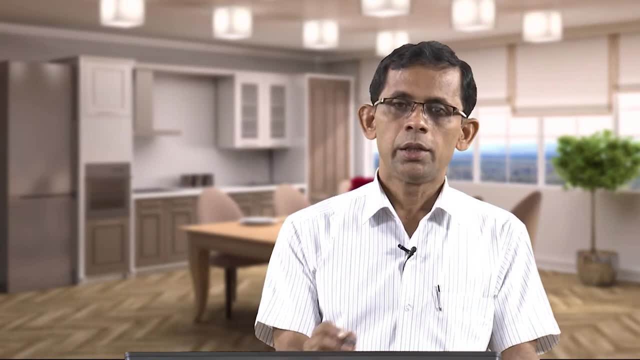 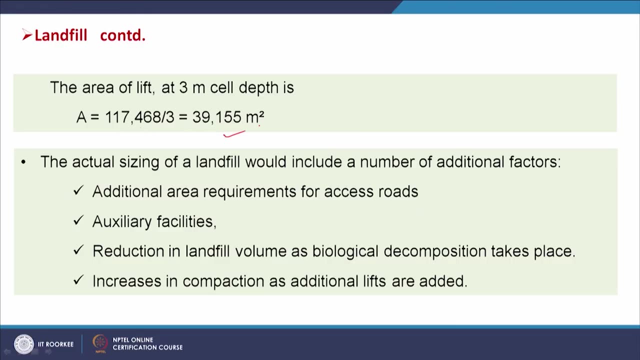 the shell depth is 3 meter. it is given so 3 into A area that is equal to volume. So A equal to volume by 3, so that is equal to 39155 meter square. So this value we are getting that is based on the mass balance, so material mass balance. but we also discuss 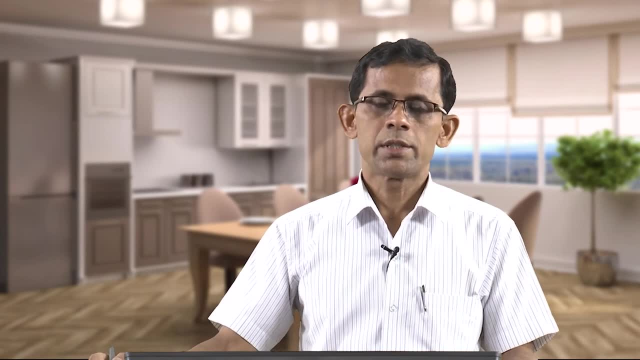 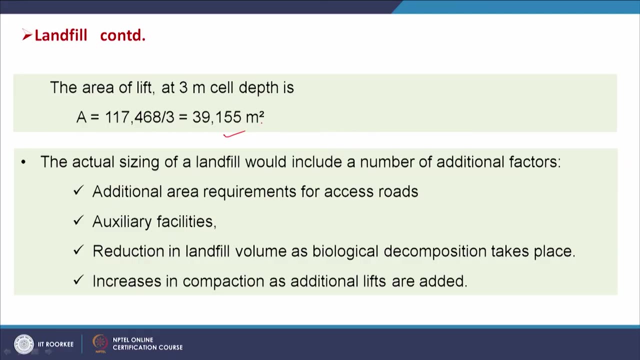 that it requires some other material, Other sites as well. this is the active filling site, but some other auxiliary areas are required, so actual size will be much more than this one. Now we will see the hazardous waste and their management. So hazardous wastes are materials. 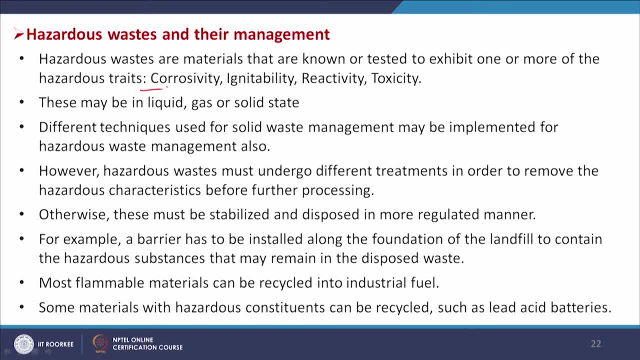 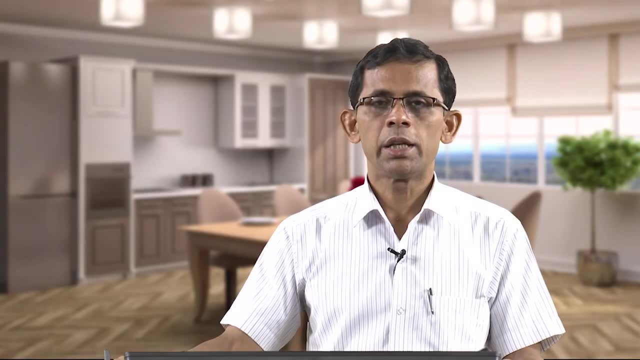 that are known or tested to exhibit one or more of the hazardous traits, that is, corrosivity, toxicity, flammability, ignitability, reactivity, etcetera. So these are the different traits. so these wastes. So these wastes have either one of these or all of these, or any two, or any combination. 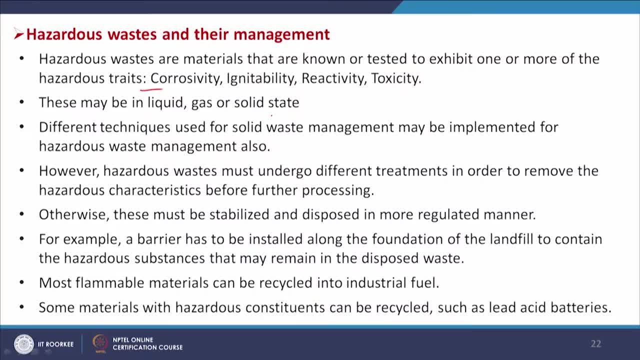 of these properties. So these may be in liquid, gas or solid state, and different techniques used for solid waste management may be implemented for hazardous waste management also. So whatever methods we have discussed, those can be implemented for this also. but there is one condition. 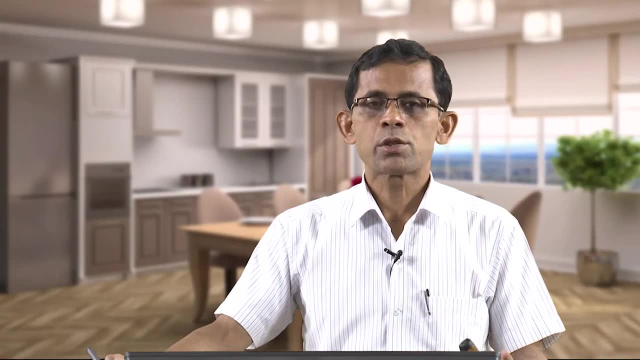 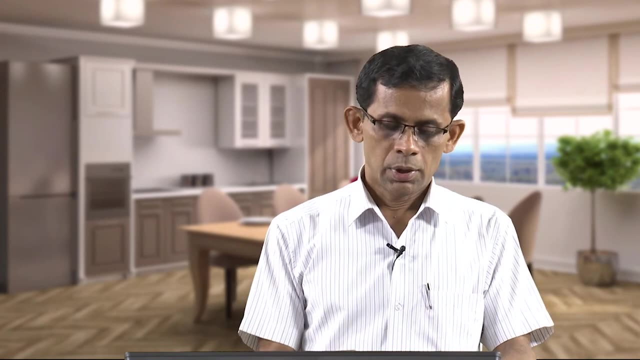 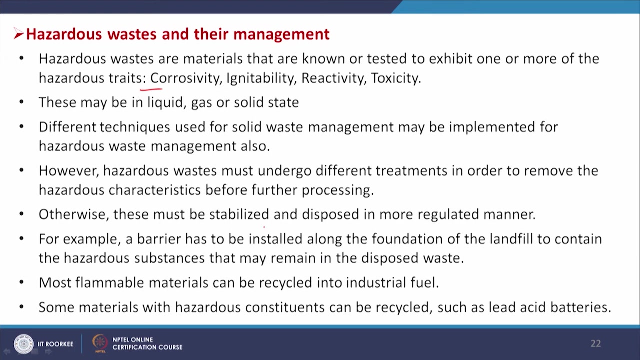 that prior using this process, it has to be decontaminated or the hazardous component has to be eliminated from it. So theAUDIOST wastewater must undergo different treatments in order to remove the hazardous characteristics before further processing. Otherwise, this must be stabilized and disposed. 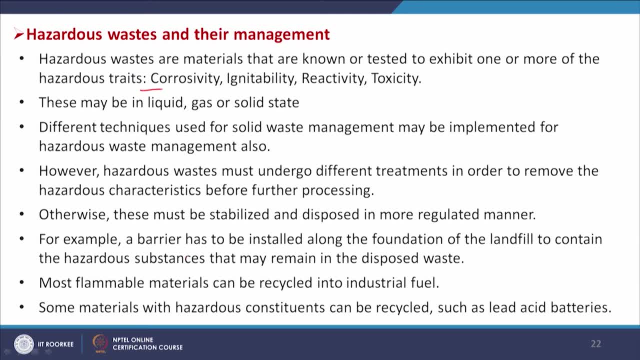 in more regular or more regulated manner. For example, a barrier has to be installed along the foundation of the landfill to contain the hazardous substances that may remain in the disposed waste. Most flammable materials can be recycled into industrial fuel and some materials with hazardous constituents can be recycled, such 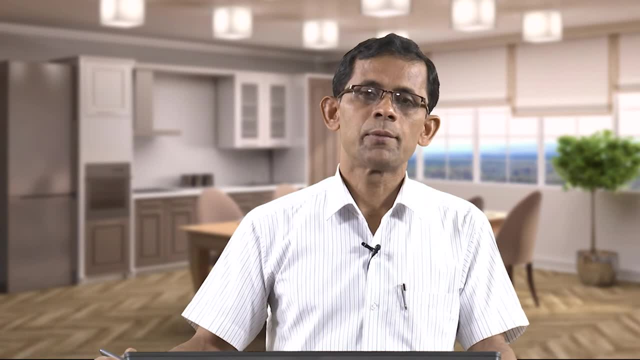 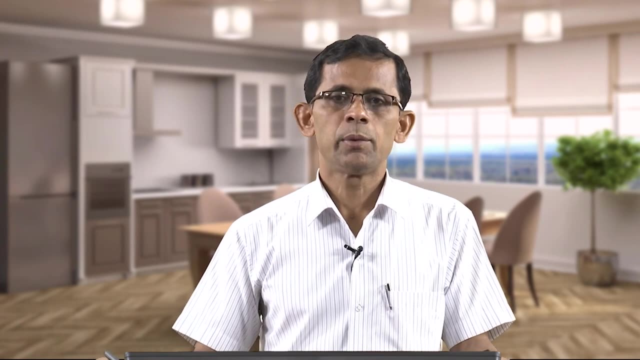 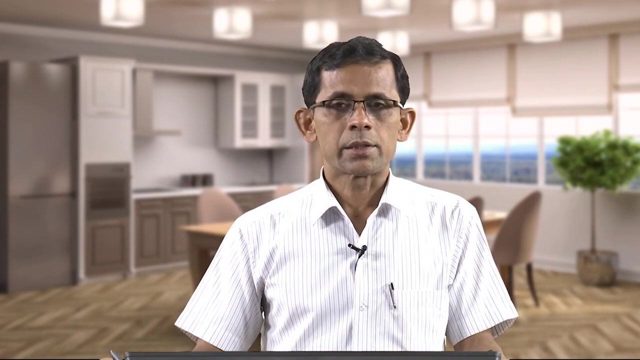 as lead acid batteries. So these are some examples of the removal of the specific characteristics from the overall waste so that the remaining part can be used following the same MSW management processes. Now we will see the waste plastics. We have seen that municipal solid waste contains good 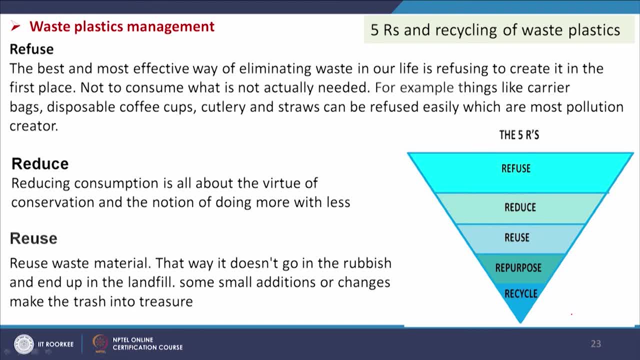 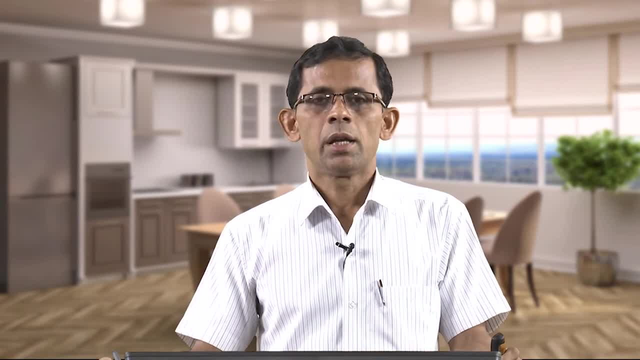 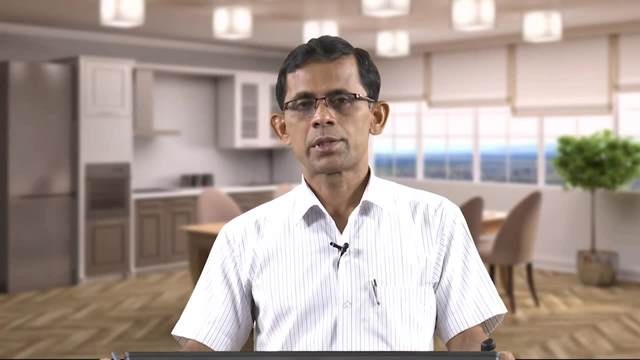 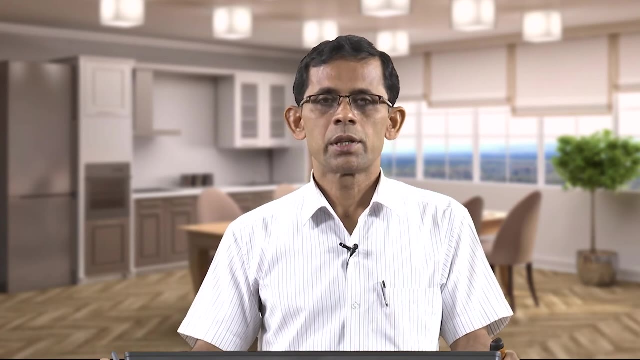 amount of waste plastics. That waste plastics can be managed by applying certain rules. The waste plastic management: certainly we can go for land filling but we can transform this part of the municipal solid waste into valuables. And the philosophy for the plastic waste management is based on the five R's. 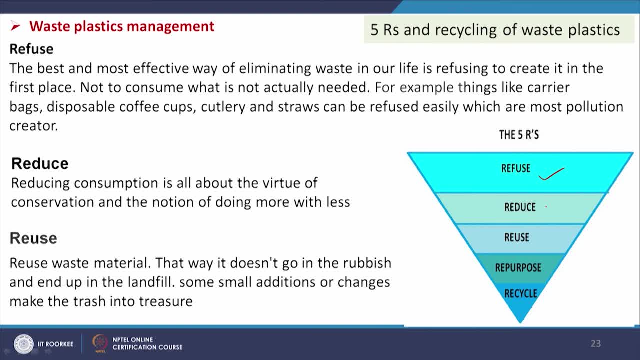 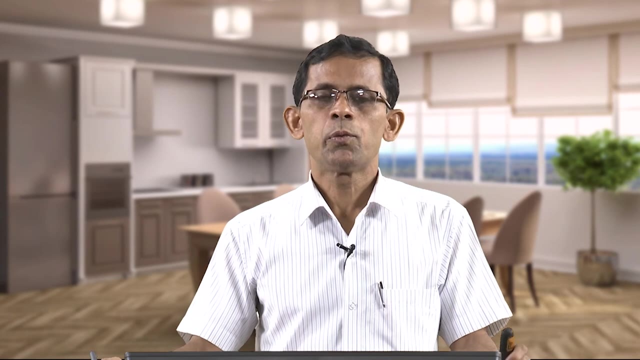 So those five R's. So the five R's are basically refuse, reduce, reuse, repurpose and recycle. Refuse means we should put our best effort not to use plastics. So, whenever applicable, we should avoid the use of plastics, For example, so when we go to shopping malls or any grocery shop. if 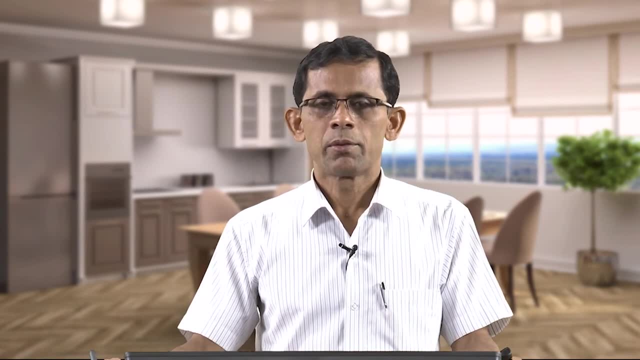 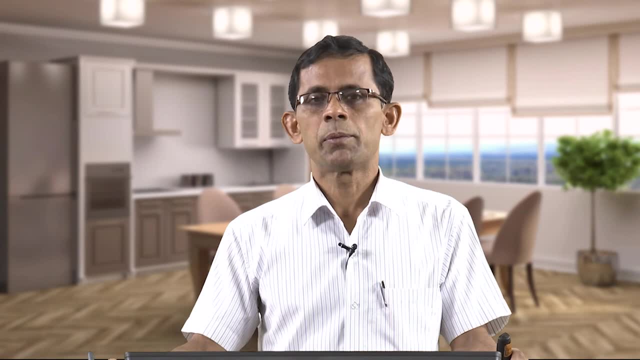 Similarly, we can ask the customer: what is the use of plastic? I do not think only其實 paper. you should carefully clean up and IVM, If we respect these two rules. For example, if plastic is nonexistent, it can take account of all of waste, like hydrocarbons. 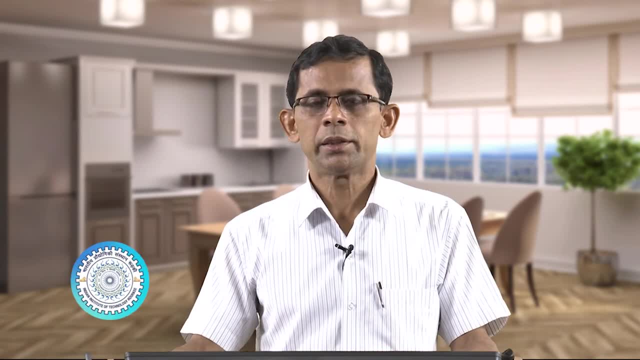 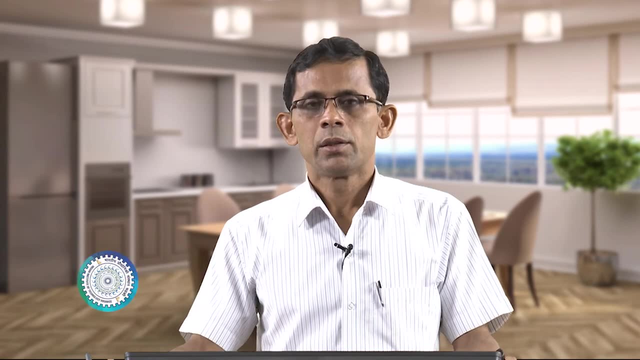 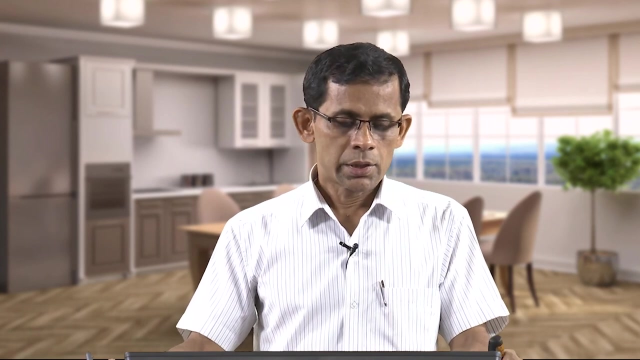 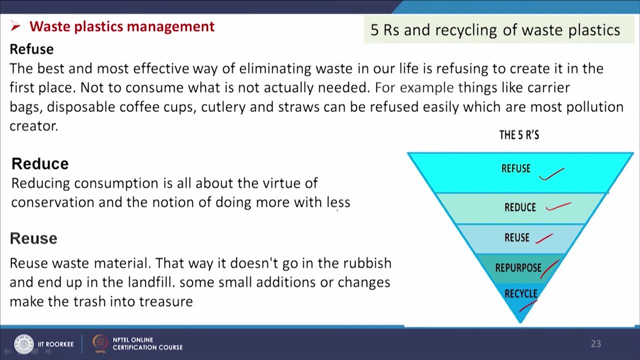 food vegetables Tages. So this is another similar type of philosophy. somewhere it is inevitable we need to use the plastic materials. but we can optimize it, we can reduce it and then reuse. reuse the waste which is being generated that can be reused. that way it does not go to the 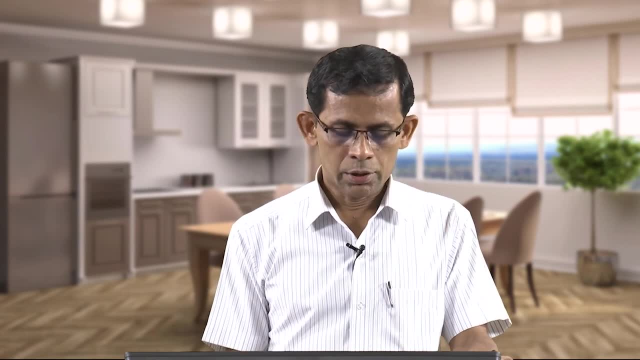 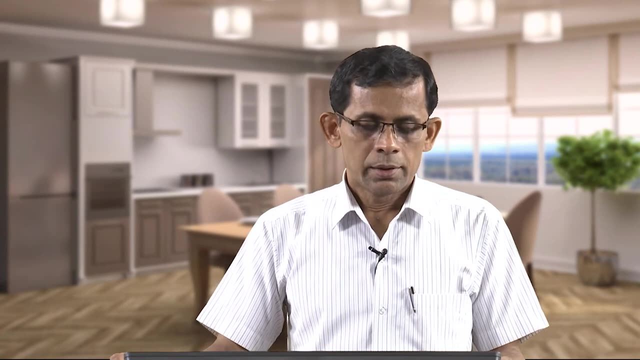 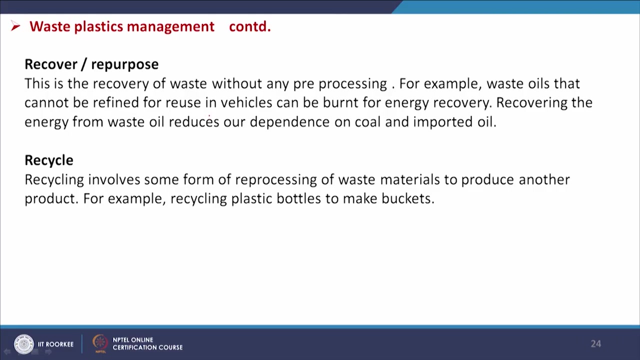 rubbish and end up in the landfill. some small additions or changes make the trash into treasure And recover. repurpose: this is the recovery of waste without any pre-processing. for example, waste oils that cannot be refined for reuse in vehicles can be burned for energy recovery. 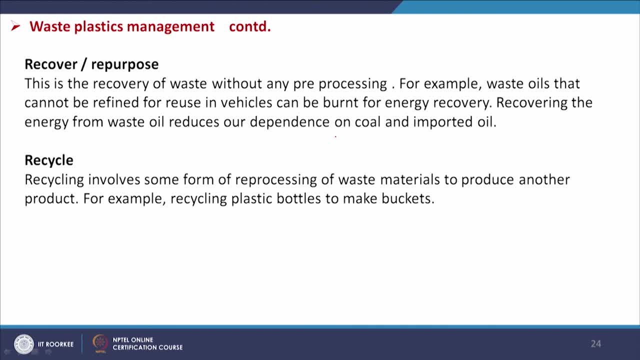 so recovering the energy from waste oil reduces our dependence on coal and imported oils. so, similar way, the plastics can be also reused, Converted to other form that can be used for other application And then recycle. recycling involves some form of reprocessing of waste materials to 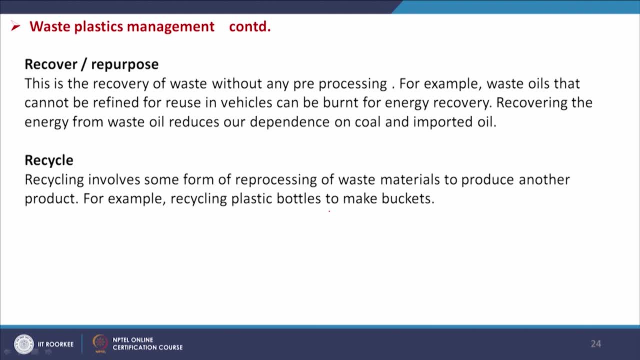 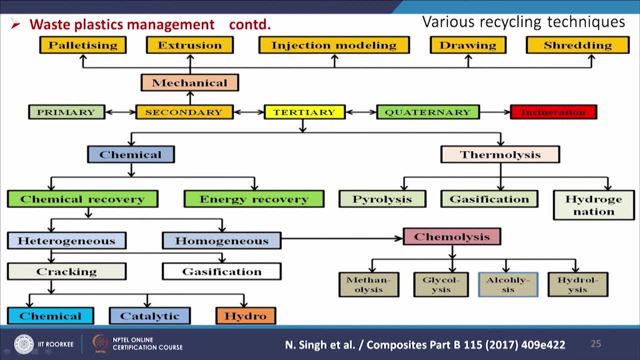 produce another product, for example recycling plastic bottles to make buckets, Now various recycling techniques which are applicable for the management of waste plastics. if we consider, then we are having, say, primary method, then secondary, then tertiary, then quaternary, So this quaternary basically incineration that is banned in the country that is not. 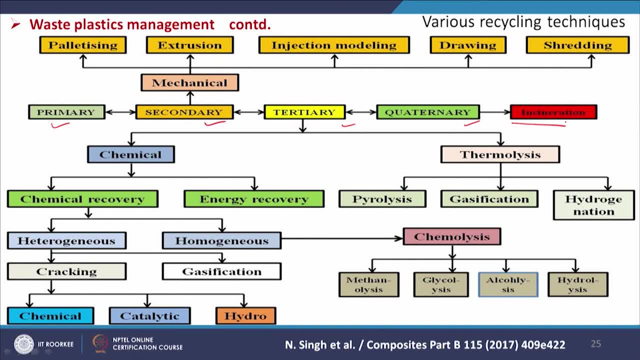 practiced and not allowed by CPCB And this secondary and tertiary are mostly favorable. primary and secondary separations is bit difficult in some time And we secondary and tertiary are main important method in the secondary, that is mechanical mildewing, Counter-inander number of Academy.